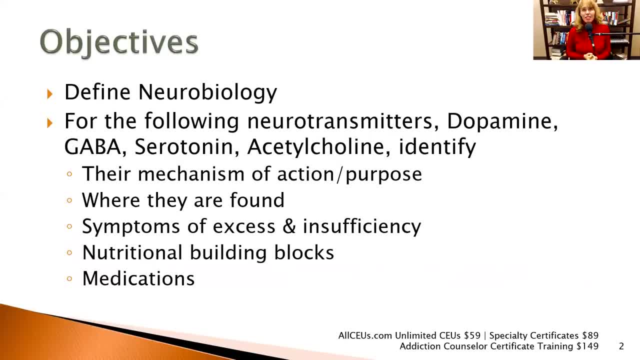 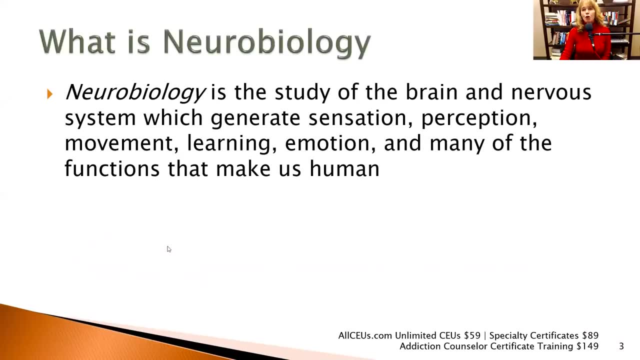 reasonable. as you'll see as we go through, really shouldn't be that hard. And then we'll look at some medications that are used to increase and decrease, or medications that may inadvertently increase and decrease the neurotransmitters in the brain. So neurobiology is the study of the brain. 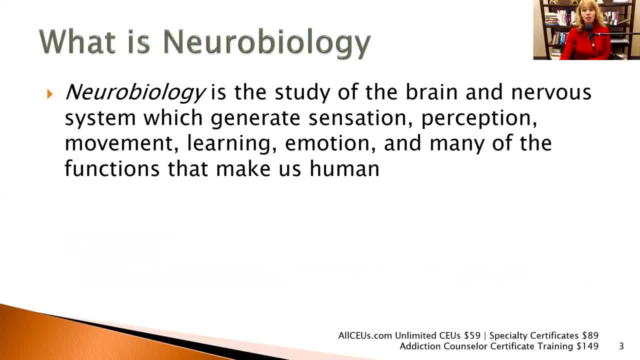 and the nervous system which generates sensation, perception, movement, learning, emotion and many of the functions that just make us human. When we have an emotion, where does that come from? Well, it's a chemical reaction that, whatever happens, kicks off a chemical reaction. And if 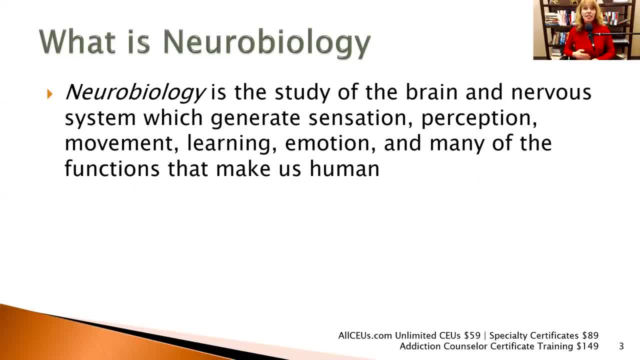 we're getting upset or getting stressed or getting excited, then we're going to have glutamate and norepinephrine and dopamine probably going out if we're excited, for example, So we want to pay attention to that. If we're calming down, then we're going to have GABA. 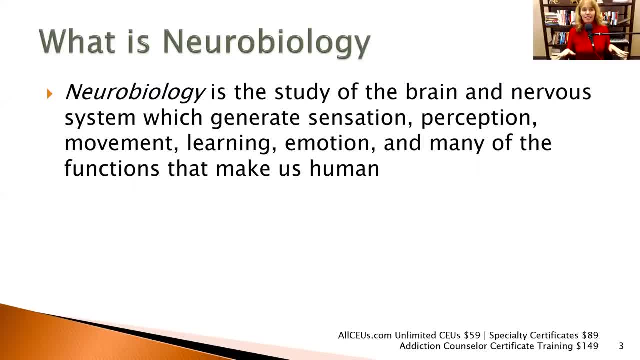 serotonin, kind of coming in and saying: all right, now's the time to rest and relax. So our emotions, or what we label as emotions, are triggered by neurochemicals. And why is that important? Well, because if somebody comes in and they're trying to address their depression, 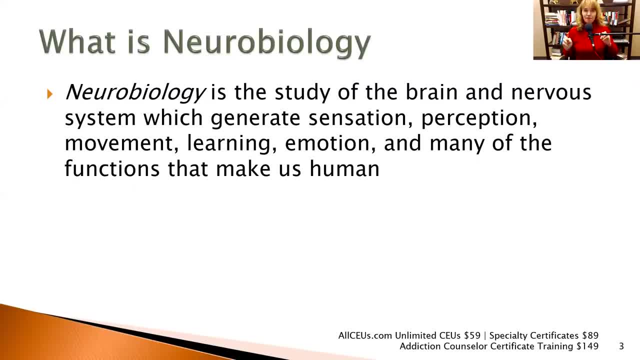 whatever that looks like for them, well that's great, But they need to understand where that's coming from. There are some cognitive things that can trigger their brain to think that there's a threat which sets off the stress response. But they need to understand that there is a. 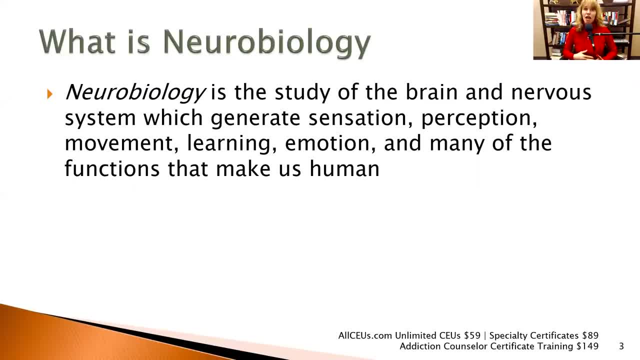 neurochemical, a biological component to it. So it's not just about changing their thinking. They also need to be making sure that their body machine is in top working order. So think about it As we go through this pre-session. we're going to talk about the 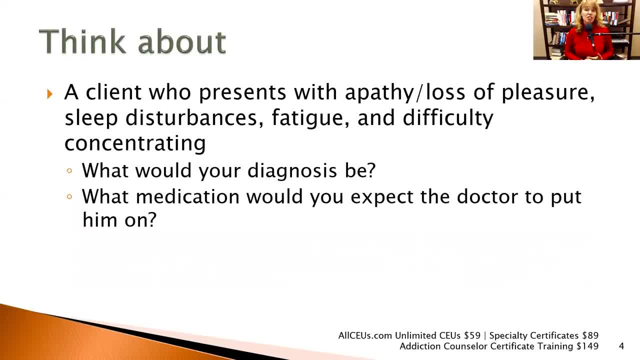 You have a client who presents with apathy, loss of pleasure, sleep disturbances, fatigue and difficulty concentrating. Yeah, my first thought is major depressive disorder or persistent depressive disorder. What would your diagnosis be? And you may say: too little information yet. 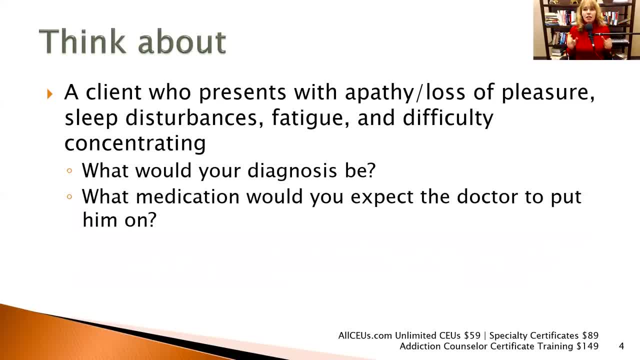 That would be a great answer too. If somebody presented to their physician with these symptoms, what medication would you expect the doctor to put him or her on? My experience has been with most physicians the first thing they do SSRIs. Let's increase. 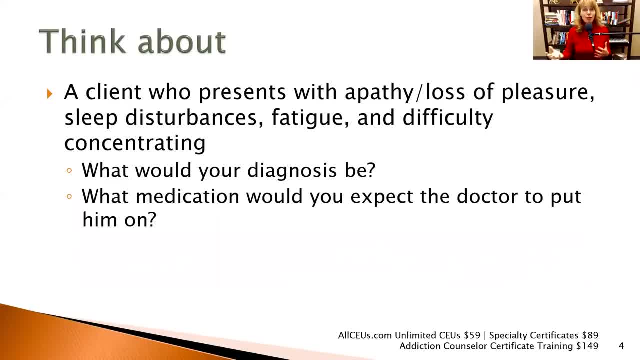 serotonin And, as you'll learn as we go through this, these symptoms are transdiagnostic and they can be caused by either too much or too little of most of the big six. So we don't necessarily know whether the person has too little serotonin. So if we start increasing it, and that's- not their problem, then we're going to have to increase serotonin. So we're going to have to increase serotonin. So if we start increasing it- and that's not their problem- then we're going to have symptoms of too much serotonin, which can be really unpleasant, And it's also whatever else was. 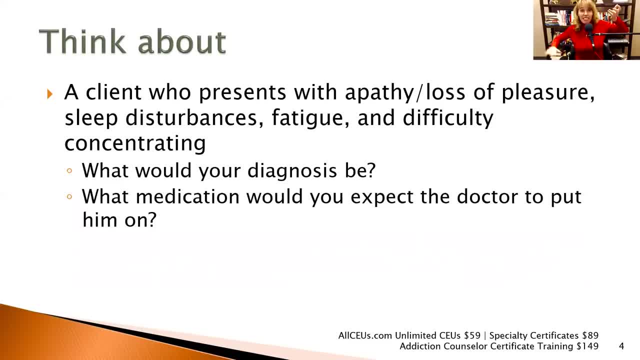 lacking down here. More serotonin means that's even more lacking, so to speak, because everything needs to be in a balance. Like I always make the analogy of a good marinara sauce, You know, if you taste it and there's not enough oregano, you know, or it's just not right and you start. 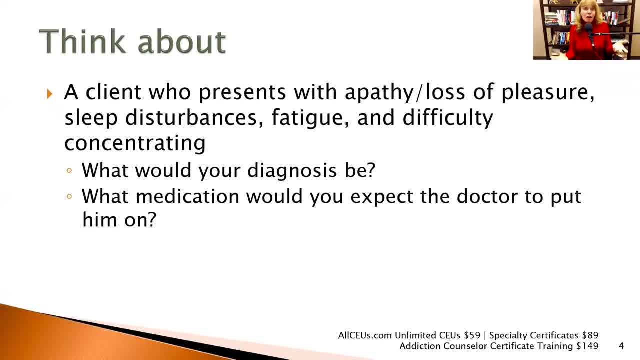 dumping oregano in. Then maybe it was garlic and not oregano, So now the oregano is even stronger and the garlic taste, comparatively, is even weaker. So we want to pay attention to what's going on And obviously 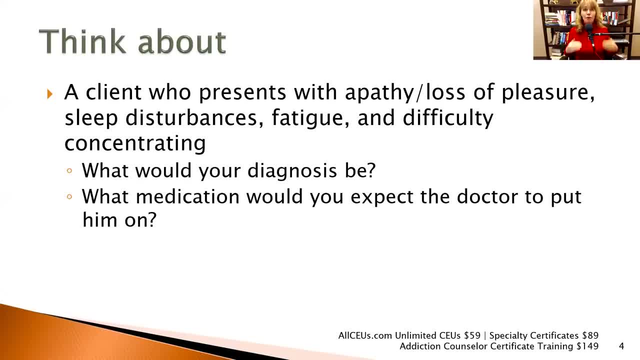 we're not making diagnoses and none of this presentation is meant to tell patients to change the medication regime or start eating a certain way or take any supplements. All of that should be covered through their primary care. So we're not making diagnoses and none of this presentation. 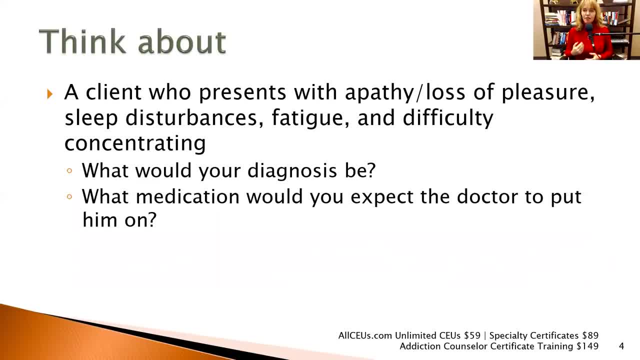 should be covered through their primary care physician, But it's important for us to be aware. So if clients are struggling because we know that antidepressants only work for 30 to 40% of the people who take them, we want to look at why is that? Well, maybe it isn't serotonin that's out. 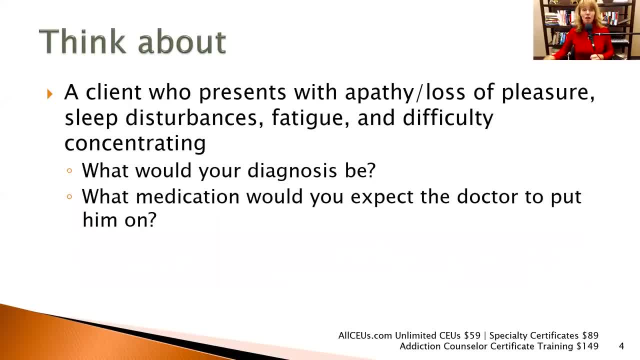 of whack for this person. Maybe there's an underlying biochemical cause, Maybe it's a different neurotransmitter, So we can help people sort of advocate for themselves. You know, maybe they need a norepinephrine reuptake And we can help people sort of advocate for themselves. 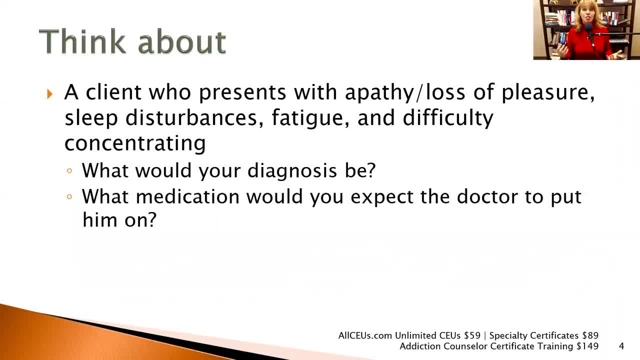 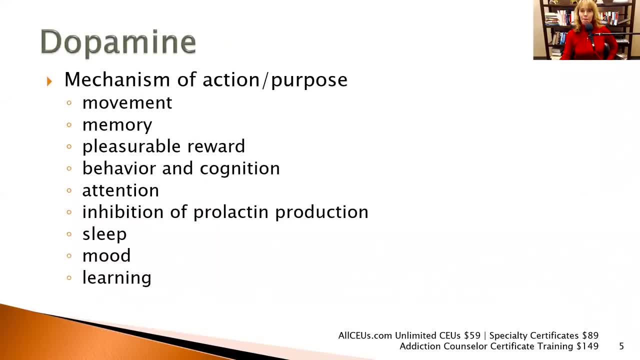 We can help them educate themselves. They need to do the advocacy and work with their physician. So, dopamine, We're going to start out with the pleasure chemical, because, well, it's first in the alphabet. No, it's not first, Anyway, it's the first one that comes to mind for most people. 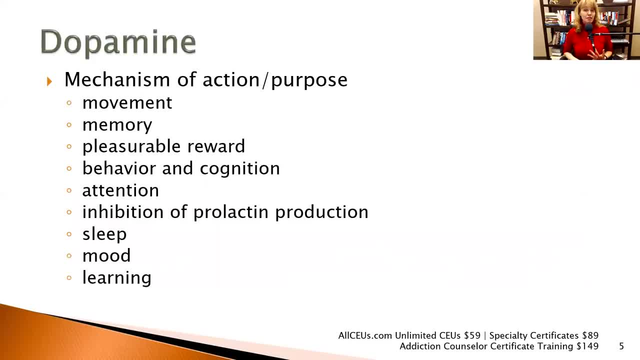 Mechanism of action. It is involved in movement, memory, pleasurable reward behavior and cognition, attention, Prolactin production, sleep, mood and learning. So it's involved in everything. So if your dopamine levels are out of whack, you're probably going to experience some difficulty in one or more of these. 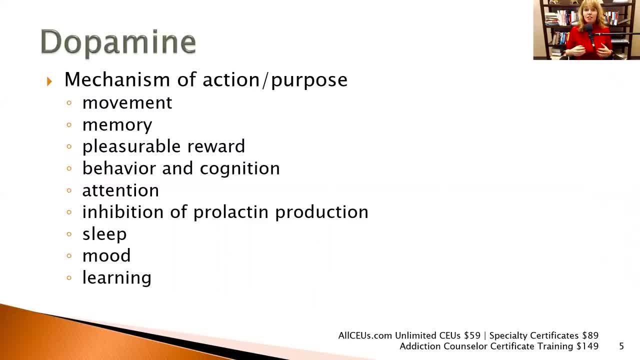 areas. Now, obviously, if you're having difficulty focusing attention, your memory is probably going to falter as well, as well as your cognition. You know you're not going to be thinking as well if your mind's racing, if you're having racing thoughts. So all of these can come together. 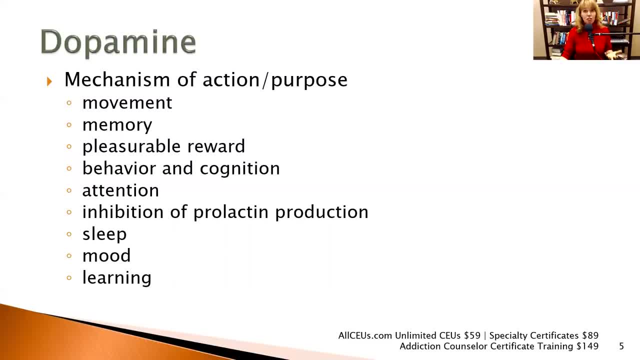 If you're not getting a good sleep. if you're not getting a good sleep, if you're not getting a good, You may start feeling sort of depressed and blue and not be motivated to focus and learn. So we want to pay attention to dopamine's impact in the person and look at our clients, who are 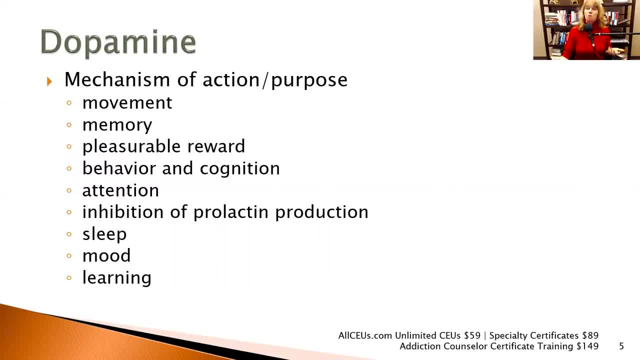 experiencing some of these symptoms that seem depressive in nature and take a look at, especially if they start on an SSRI or they've been on them before and it hasn't worked. You know we may want to look at. is there something else that we can do? Is there something else that we can do? Is there? 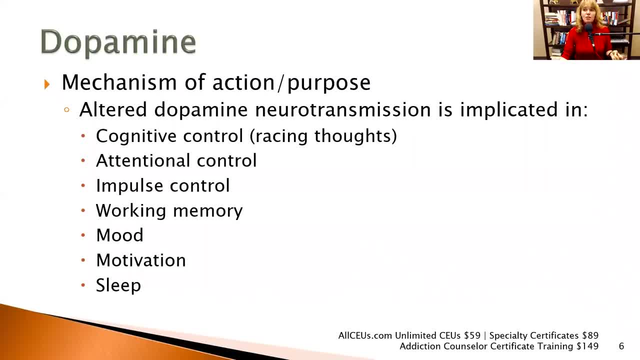 something else that's causing it: Altered dopamine neurotransmission. So if you're not getting enough or you're getting too much cognitive control, people will have racing thoughts. Attentional control can't focus, Impulse control, self-explanatory Working memory is going to kind. 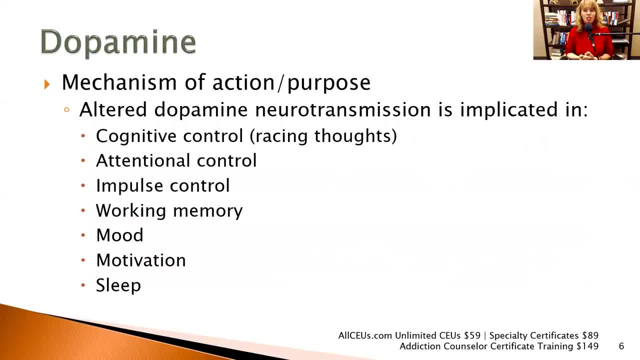 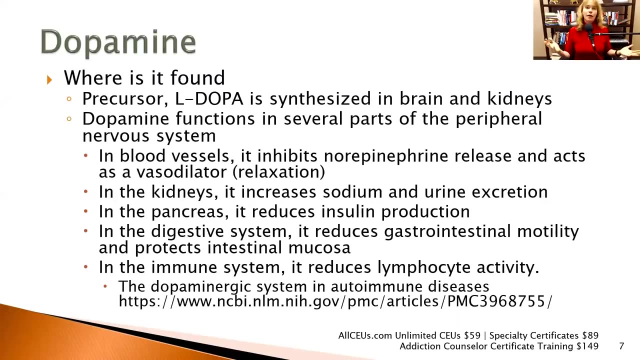 of go, which you would expect with problems with attentional control and racing thoughts. Mood, motivation and sleep are all going to be impacted. So where is dopamine found, You know? okay, we realize that there may be a problem with it- Where? 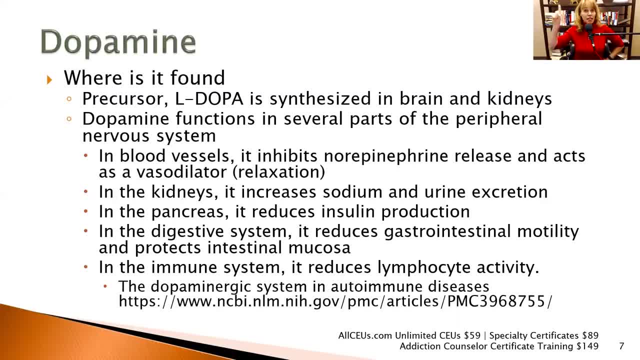 do we find it? Well, it's in the brain and the kidneys- Kidneys. So if you have a client who has kidney disease or is taking any kind of medication that alters kidney functioning and or maybe engaging in high-intensity activities that are causing fluctuations in hydration, it can alter. 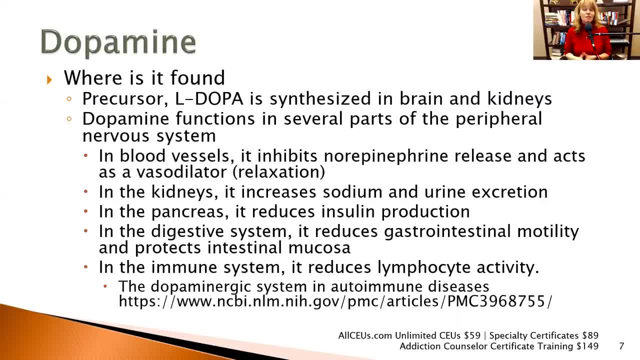 to a certain extent, dopamine levels Definitely can alter medication levels. Dopamine functions in several parts of the peripheral nervous system. In blood vessels. it inhibits norepinephrine, which is our motivation and focus chemical and excitatory chemical, And it acts as a vasodilator, So it helps us relax. 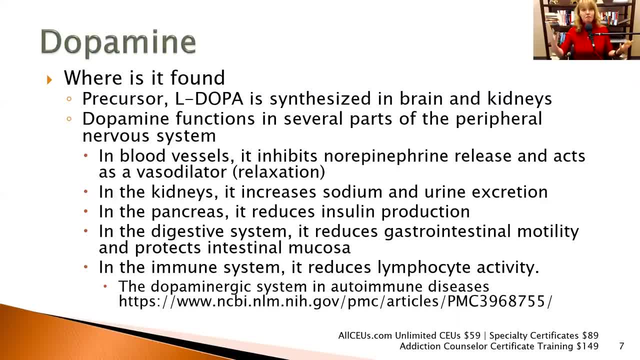 So if you have a client who's kind of stressed high-strung dopamine, may be part of it. In the kidneys it increases sodium and urine excretion. So it keeps the kidneys functioning well And if you don't have the right sodium balance you can have something called rhabdomyolysis. 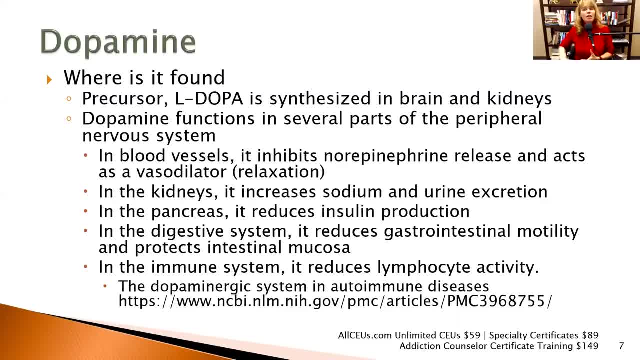 which can be really bad. So we want to make sure that clients are going to the bathroom enough. In the pancreas it reduces insulin production. If we're working with a client who is diabetic, paying attention to their moods, their sugar levels and all of that may be important And 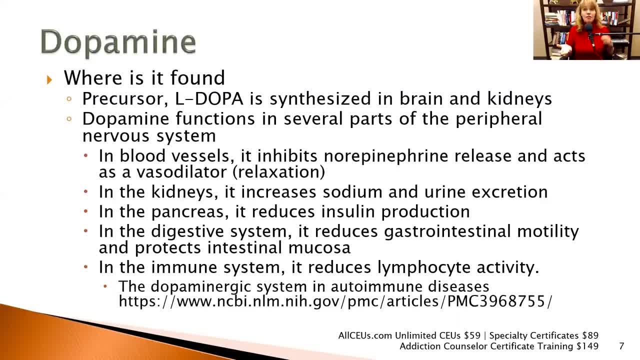 if they're having difficulty stabilizing their sugar levels, they may be able to do that. Looking maybe at dopamine In the digestive system, it reduces gastrointestinal motility and protects the intestinal mucosa, So it slows things down In the immune system. 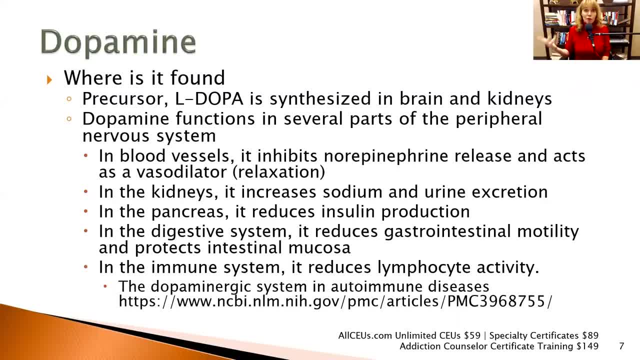 it reduces lymphocyte activity. So why do we care? We're mental health Because it can be implicated in autoimmune diseases, And I've linked to several articles through here that have indicated that if dopamine is increased, they found that it can be used to reduce the amount of dopamine that's in the body. So if you're 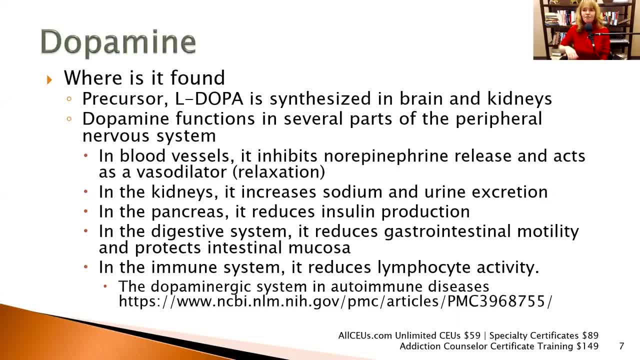 an increase or is decreased. I'm sorry. they found an increase in lymphocyte activity. So people who have autoimmune diseases may not have enough dopamine. So if dopamine is increased then that lymphocyte activity, that overactive immune system, is blunted sometimes. 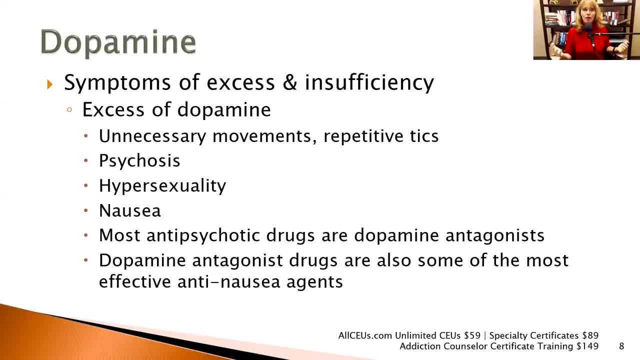 Symptoms of excess, And when we think about dopamine, one of the first things we often think about is schizophrenia. Not necessarily the only thing that we think about is schizophrenia, And we don't know that dopamine problems actually cause schizophrenia. Because when we address schizophrenia with dopamine antagonists or dopamine agonists- depending on whether you're- 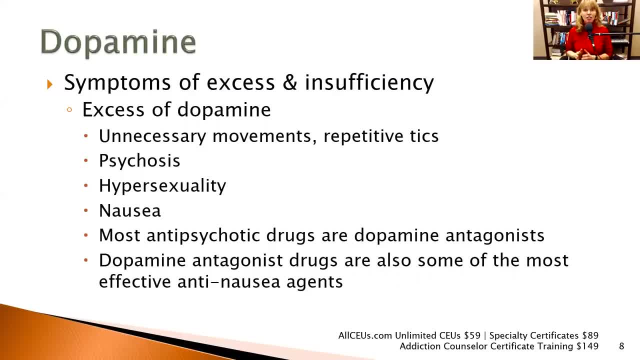 looking at positive or negative symptoms, it only partially addresses the problems people are having, And then the side effects are horrid. There are other medications- and I'm getting ahead of myself- that also produce psychotic-like features. So we're not for sure whether dopamine is it. We think dopamine's involved, But there are probably. 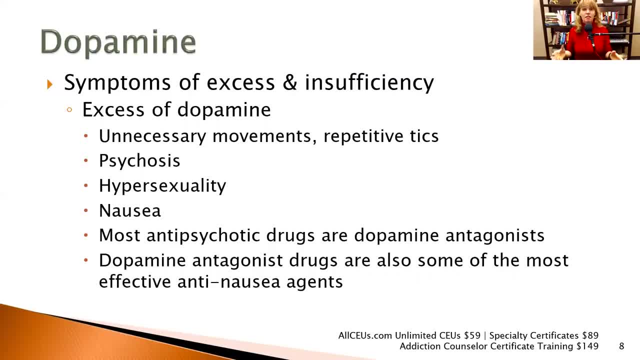 other neurochemicals that are also involved in the development of schizophrenia. So too much dopamine, Unnecessary movements, repetitive tics, psychosis, hypersexuality, nausea- This can also kind of overlap a little bit with hypomania or mania If you've got somebody who is really you know. 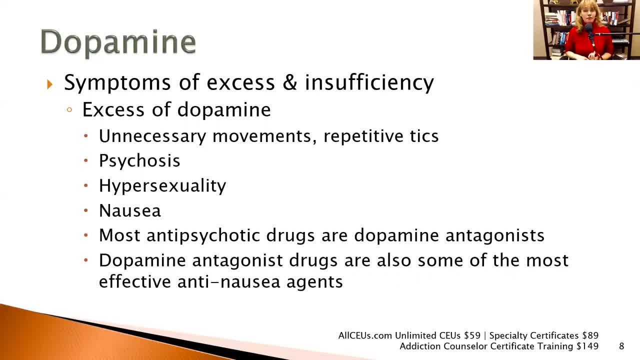 physiologically agitated- and they may with mania- they're going to have some psychotic features. There's hypersexuality is common, So these are all common in when there is too much dopamine. Most antipsychotic drugs are dopamine antagonists, So they're going to make these things. 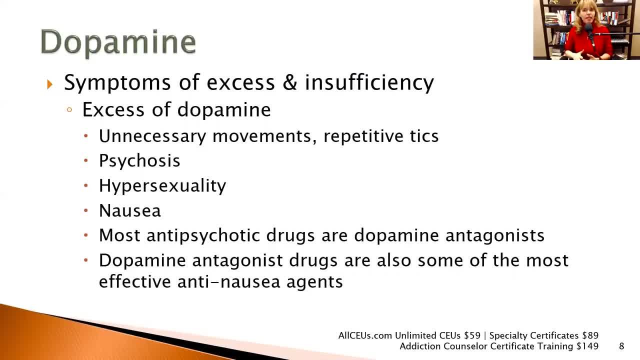 go away. They're going to slow the person down, get rid of the psychosis, reduce the sexuality, reduce the nausea, in order to bring it back in line with what the person wants as a quality of life. Dopamine, antagonist drugs are also some of. 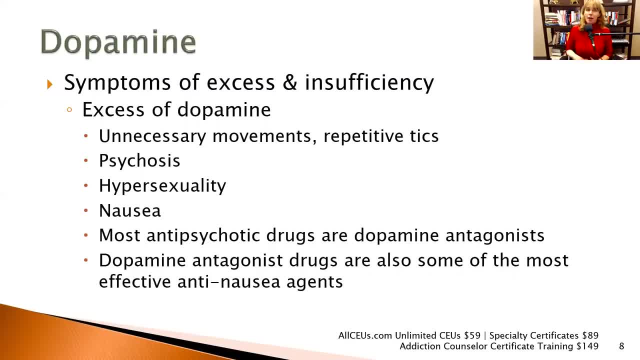 the most effective anti-nausea agents. If you have somebody who's going and going out on a boat, on a cruise and they're going to, they're afraid they're going to be seasick and they start taking anti-nausea agents. Women who are pregnant sometimes take anti-nausea agents if they 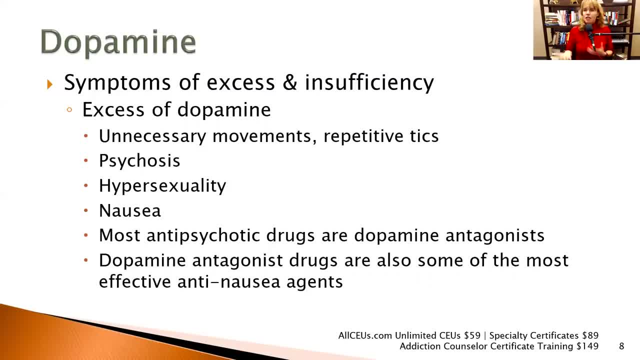 have really bad morning sickness. So there are a lot of times where you may see this used. When my son was got out of the NICU, he had gastric esophageal reflux disease and they prescribed him Reglan, which I didn't realize at the time. how powerful of a 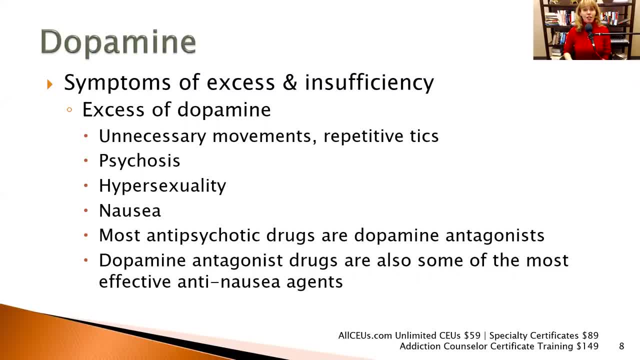 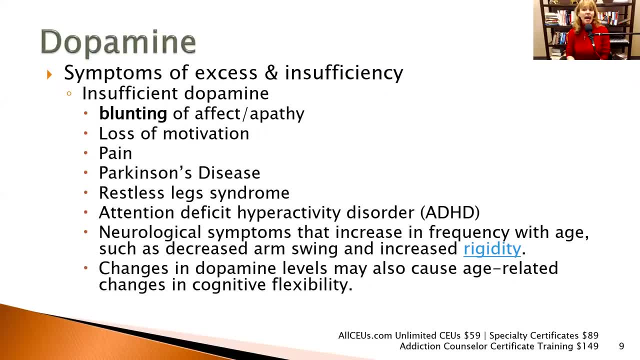 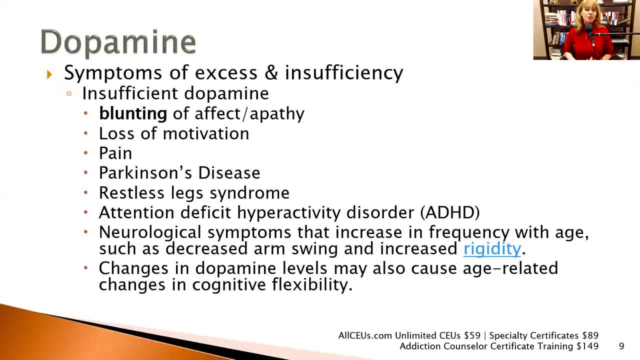 motivation, increased pain, symptoms of Parkinson's disease or restless leg syndrome, attention deficit, hyperactivity disorder, because dopamine helps us focus. neurological symptoms that increase in frequency with age, such as decreased arm swing and increased rigidity, And changes in dopamine levels, may also cause age-related changes in. 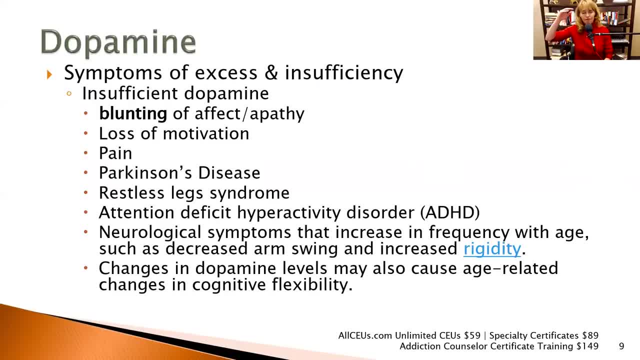 cognitive flexibility. So as dopamine goes down we lose some cognitive flexibility. But thinking again, if we have a client who has normal dopamine levels and they start taking a powerful anti-nausea agent for some reason and they start feeling sort of depressive symptoms, or 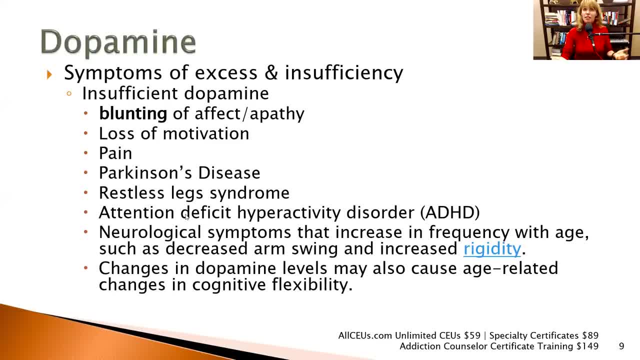 restless legs or ADHD type things. we want to try to connect the dots as a side effect of that- potentially a side effect of that anti-nausea agent that they may need to talk over with their doctor If they didn't have the symptoms until they started taking the medication. 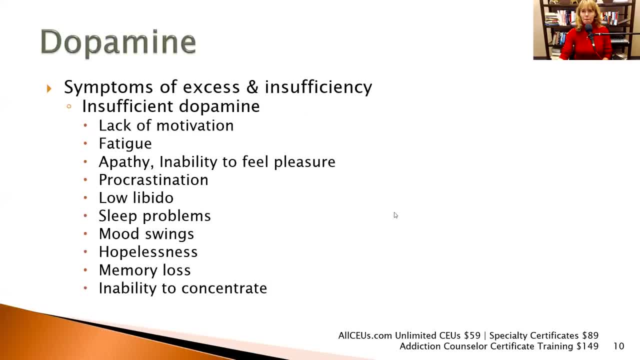 and then all of a sudden they're having them. Other symptoms of insufficient dopamine: lack of motivation, fatigue, apathy, procrastination, low libido, sleep problems, mood swings, hopelessness, memory loss and difficulty concentrating. I think I covered those on the other slides leading up to this, But a lot of this. 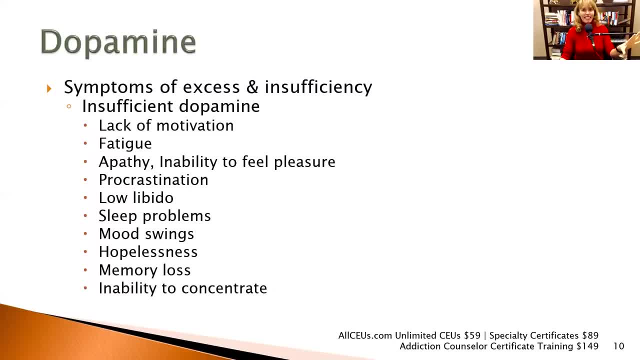 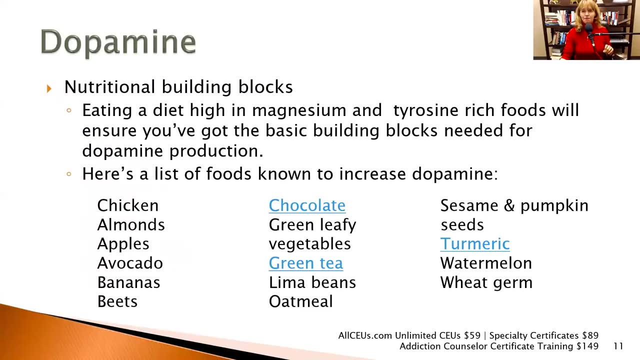 looks like on a quick glance. looks like depression, which again, a lot of times, doctors are going to go straight for a selective serotonin reuptake inhibitor. So that might not be the best thing for that person. Nutritional building blocks, Eating a. 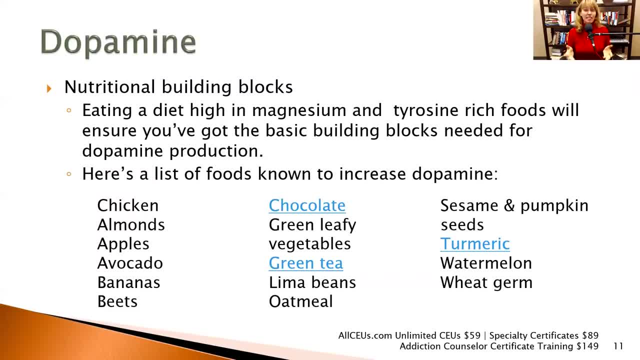 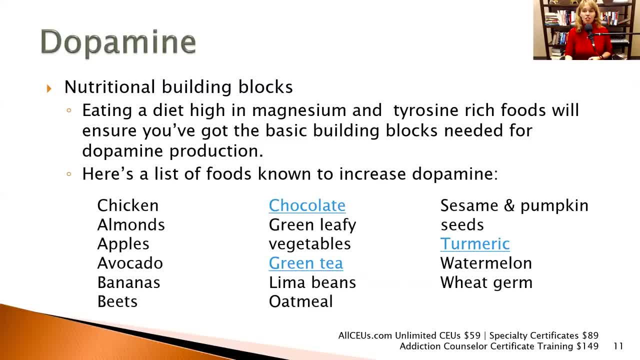 But it ensures you've got the basic building blocks needed for dopamine production: Chicken, almonds, apples, avocados, bananas, chocolate. I like chocolate And you know you can get the chocolate powder, the Hershey's cocoa dark chocolate powder. 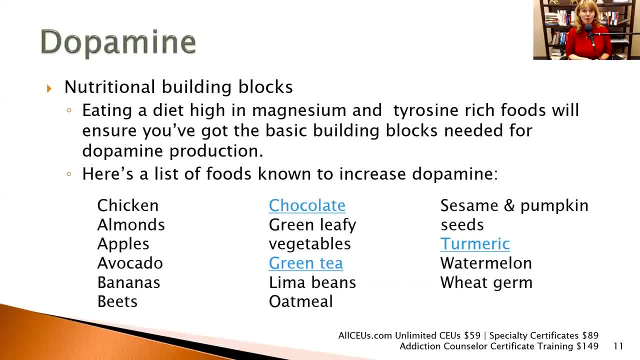 And it has, like I think it's- 10 calories per tablespoon, So it's not the same as eating a chocolate bar. So if people are trying to increase their chocolate consumption, that's one way to do it where they're not getting all those saturated fats and everything. 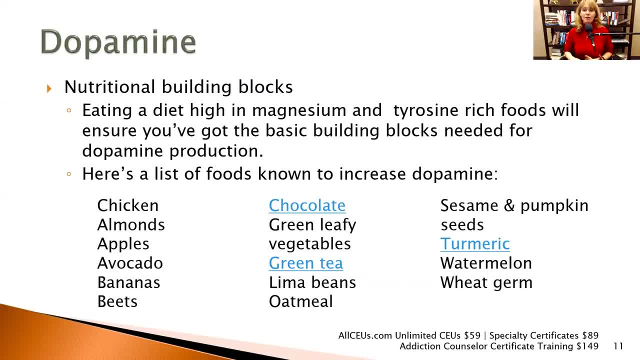 And green leafy vegetables, green tea, lima beans, oatmeal, sesame and pumpkin seeds. turmeric, which is a spice. You're not going to eat enough turmeric to really increase your dopamine levels unless you're really experimenting with your cooking. 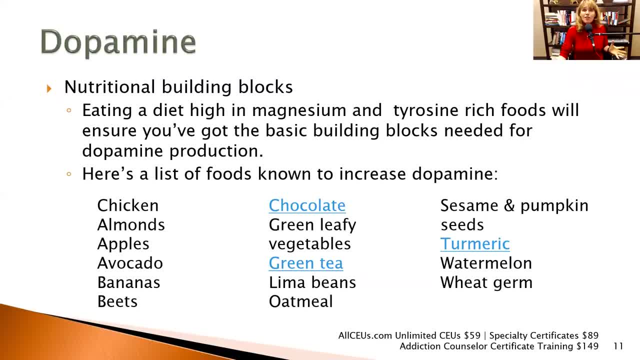 Watermelon and wheat germ. So most people can find two or three things on this list that they're willing to eat, And you know. that's all we're talking about. We're not talking about anything huge in terms of altering Their diet. again, they need to talk it over with their nutritionist. 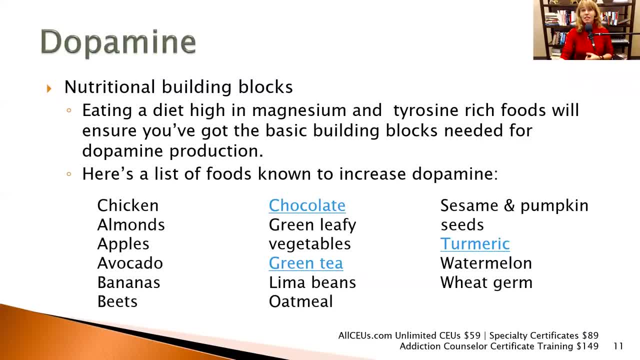 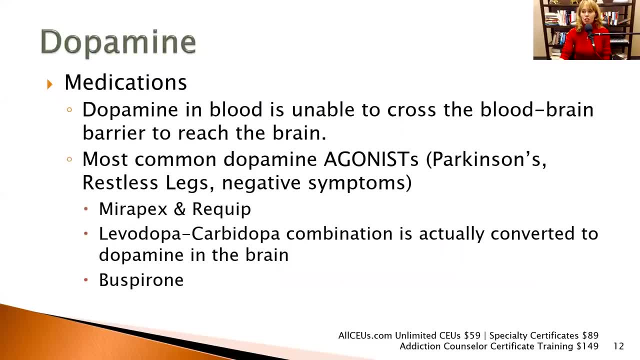 If they're on any sort of medications, especially MAOIs or typical antipsychotics, it's going to be even more important that they talk with their nutritionist or physician, because there's a lot of dietary restrictions with those medications. Dopamine in the blood is not able to cross the blood brain barrier to reach the brain. 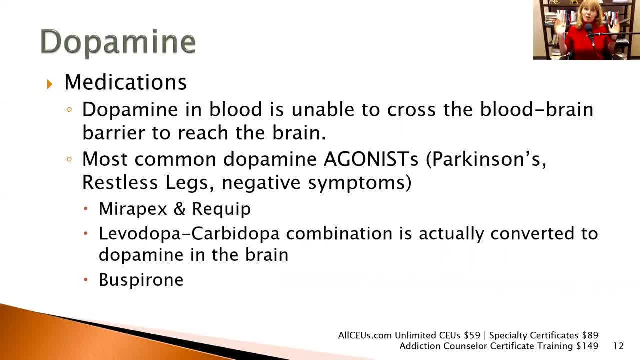 So people can't just take a supplement of dopamine and go, okay, Cool, I'm good. So they need to have provide their body the building blocks so their brain can make the dopamine, The most common dopamine agonists. So this is what increases dopamine and is going to get rid of negative symptoms, which 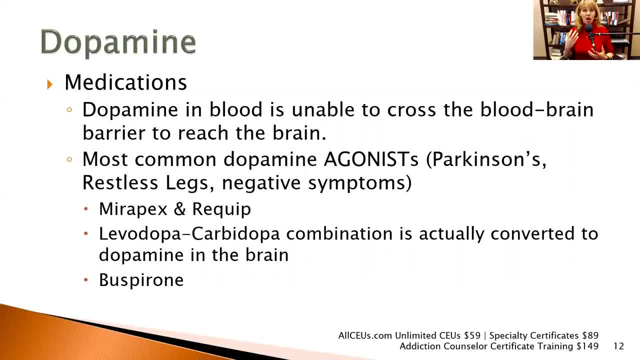 are your apathy, your depressive type symptoms. You're not wanting to speak, your catatonia. restless legs, Parkinson's? Mirapax and Requip are the name brands of two of them, The more common medications that are prescribed: levodopa, carbidopa and there's. that's the 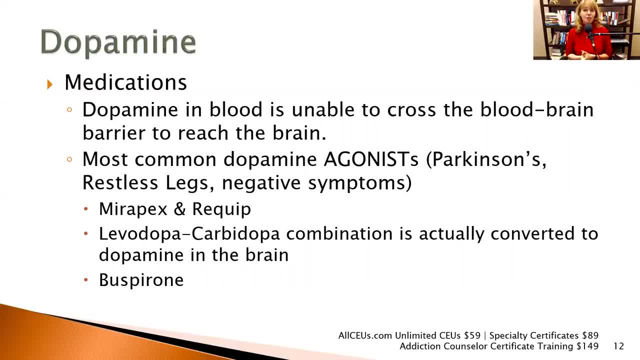 generic is converted to dopamine in the brain. So that's another drug that they often prescribe, but a side one to consider, And a lot of our clients are on buspirone, So a side one to consider and just to learn a little bit about is buspirone, because it 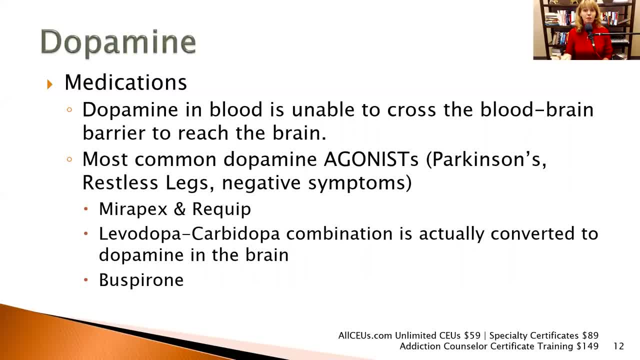 does increase freely available dopamine in the brain And in the brain. So that might be one. It's not nearly as powerful as the other two, but it might be one that our clients look towards. If you're not familiar with buspirone, it's not a benzodiazepine or a barbiturate, but 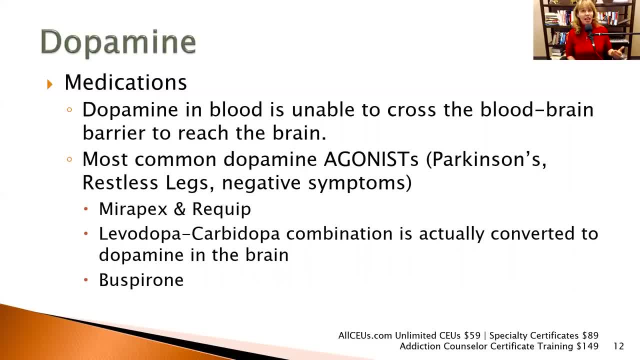 it has a lot of anti-anxiety type properties. It's one that takes time to get into the system like an antidepressant- takes two to four weeks to build up in the system, But it's non Addictive in the same way you know it's. it's not addictive like Xanax or Valium or 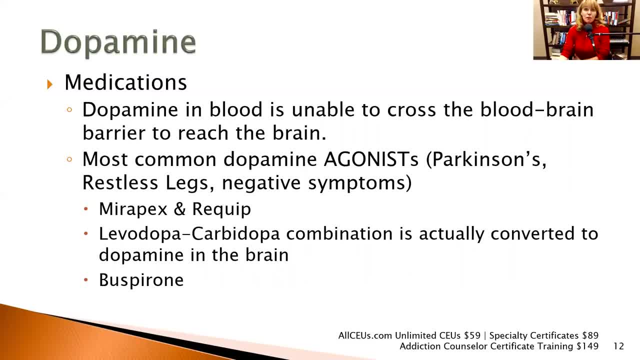 any of those are. So it is one option, especially for clients who have co-occurring issues, that they can consider for anxiety If some of the other things make them too tired, like some of the antidepressants that are also used for anxiety at high levels. 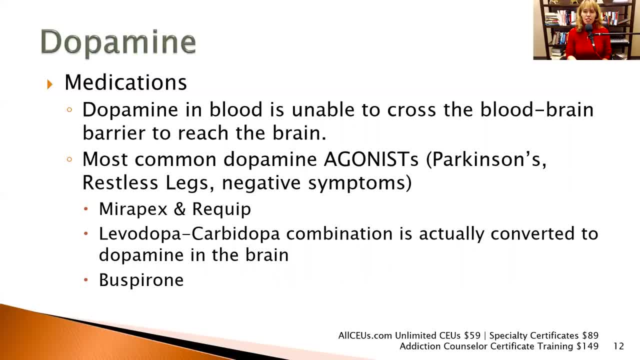 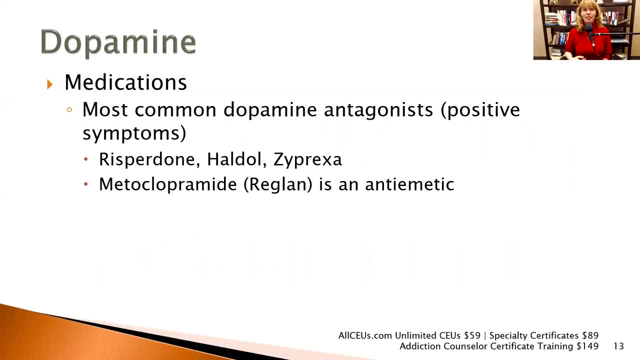 And what's the other one? I was thinking of Seroquil. That's another one I've seen prescribed for anxiety. So so these are options for them. Most common dopamine antagonists: These are the ones that get rid of the positive symptoms such as the hypersexuality and nausea. 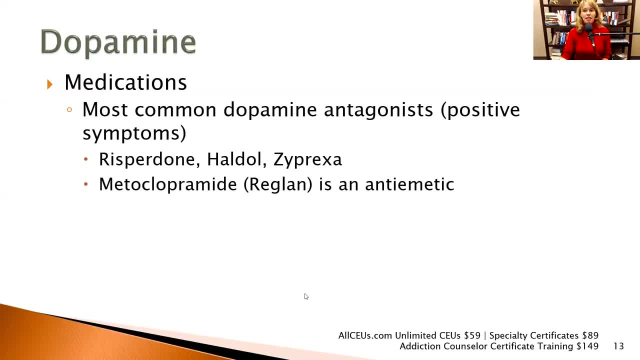 and things like that- Risperidone, Haldol and Zyprexa. They will also get rid of the hallucinations, the delusions, things that you don't want to be there, that are there. Reglan is the one I told you about that. um, metoclopramide is an anti-nausea medication. 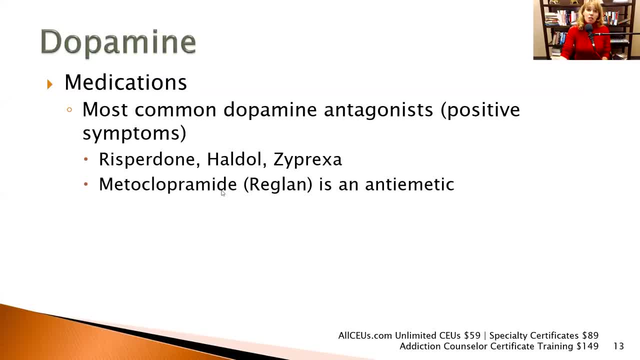 And it also helps speed up gastric emptying. So some of your clients, especially your elderly clients who are, or people who have gastric esophageal reflux disease, GERD, um- may be on this, So being aware that this, uh, this medication will blunt and slow people down a little bit. 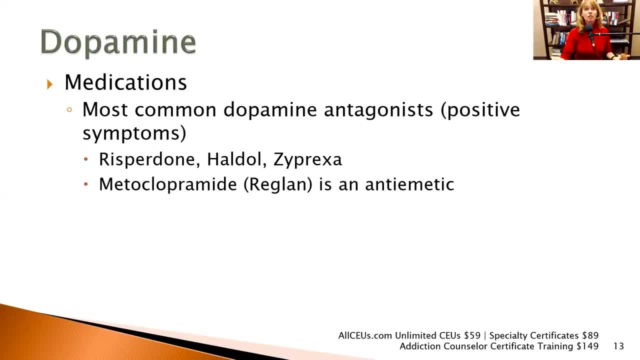 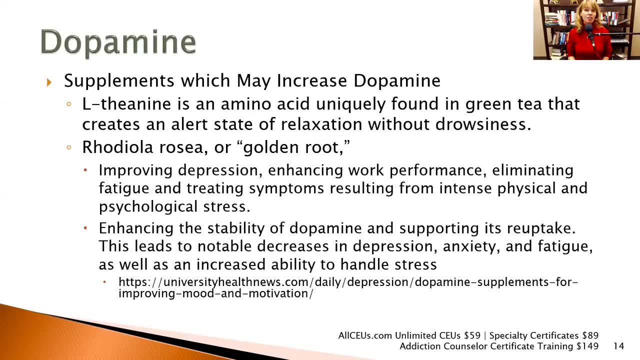 So if they're starting to feel depressed, um, take a look at side effects of medications, Supplements which can increase dopamine. L-theanine- It's another amino acid that's found in green tea, So if people are just drinking green tea, they're not going to get enough L-theanine. 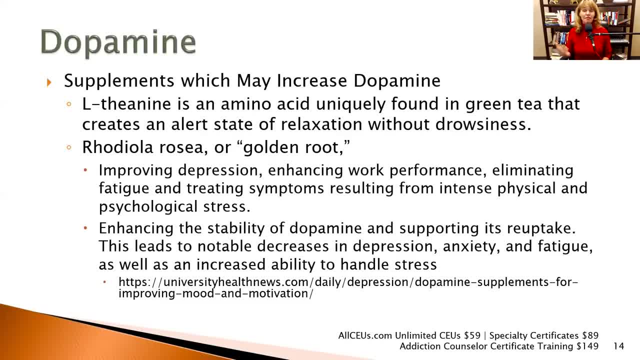 to you know cause any problems or negative interactions with their medication, but you can get it as a supplement. So if clients are talking about taking this as a supplement, especially if they're taking other um psychotropic meds, they need to let their doctor know. 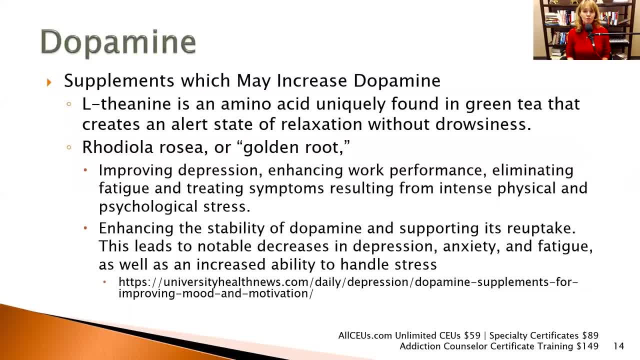 Rhodiola, Rhodiola rosea or golden root, also increases dopamine uh by enhancing the stability of it and supporting its reuptake, which has been shown to produce decreases in depression, anxiety and fatigue and an increased ability to handle stress. 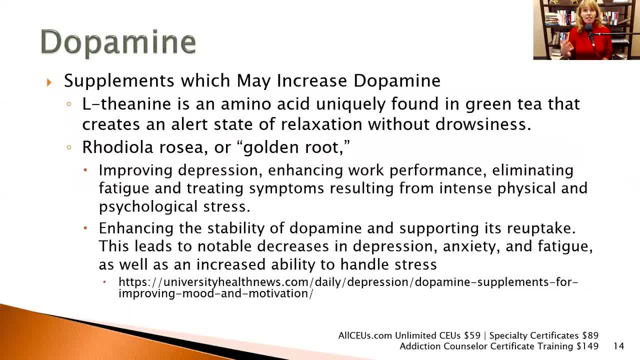 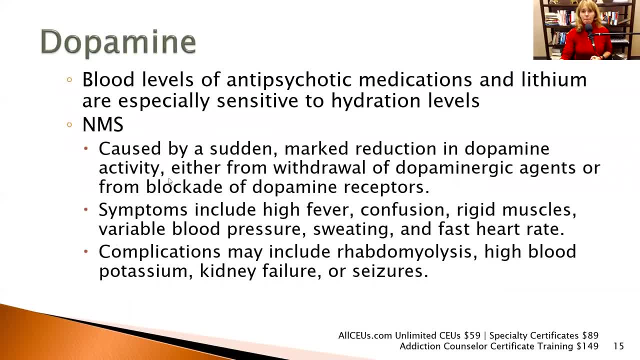 So it's an herb that's used a lot in Eastern medicine in order to provide anti-anxiety, antidepressant type effects. Blood levels of antipsychotic medications and lithium are especially sensitive to hydration levels, So if your client is taking any of those, it's important that they are aware of, uh aware of this fact that they 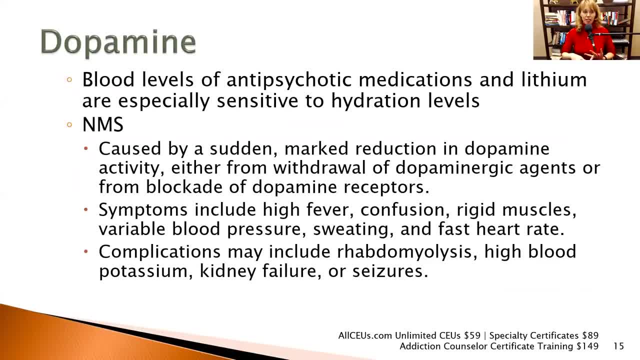 don't get too dehydrated, but they also don't get too hydrated. Um neuro, uh. neuromalignant syndrome is caused by a sudden marked reduction in dopamine activity, either from withdrawal of dopaminergic agents or from blockade of dopamine receptors. 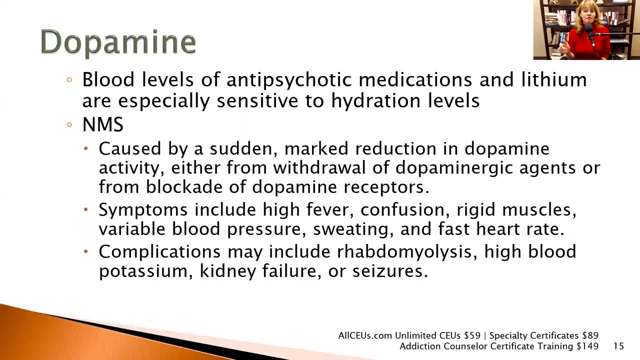 Symptoms include high fever, confusion, rigid muscles, variable blood pressure, Sweating and fast heart rate. Now, this is also very similar to the symptoms that you're going to see when we talk about serotonin syndrome, So it's important to pay attention when these symptoms are there, because it's life-threatening. 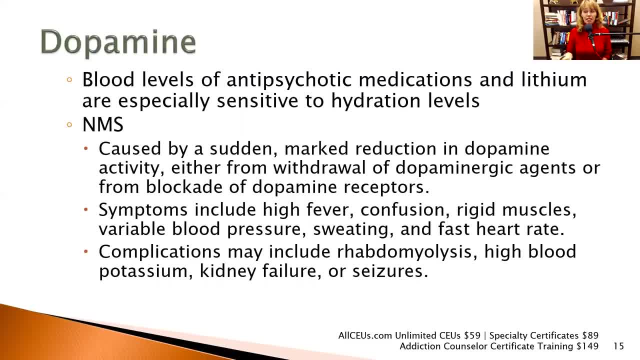 Um, complications can include rhabdomyolysis, the kidney problems, high blood, potassium, kidney failure or seizures. Um, so we want to be aware of what's going on with our clients. Uh, we want to talk with them about any symptoms that they're. 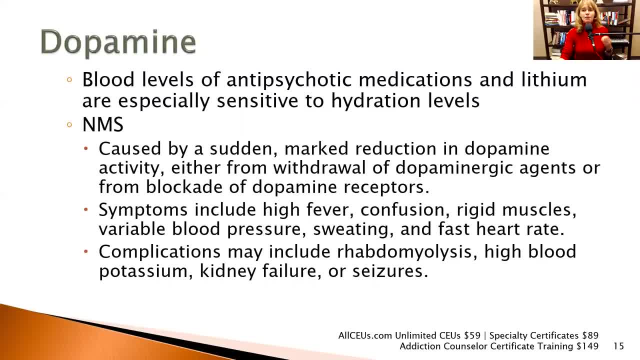 having. This can be caused, you know, by any sort of sudden reduction, And it doesn't have to be just from um, a reduction in in a dopamine-type medication. They've shown it with some other um medications as well. 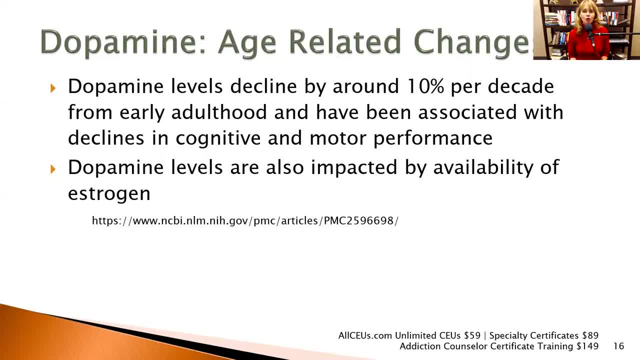 Dopamine levels decline by around 10% per decade from early adulthood and have been associated with declines in cognitive and motor performance. Dopamine levels are also impacted By the availability of estrogen. So here's another age-related change. If you're working with a woman who is older, a woman who is, uh, experiencing premenstrual, 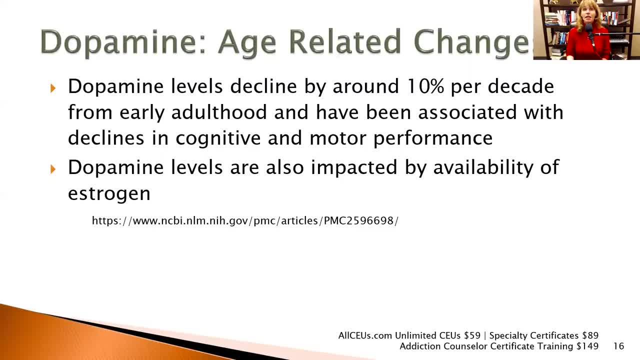 dysphoric disorder, a woman who is recently postpartum, it's important to look and realize that hormone levels are fluctuating widely, which also means dopamine levels are going to fluctuate widely. Um, as far as Welbutrin as an agonist, I'm not aware. 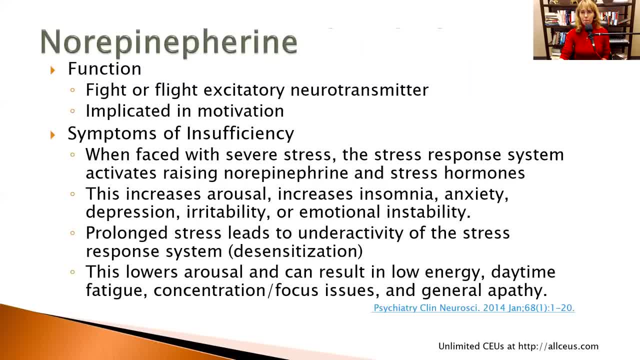 I? I don't know the answer. I don't know the answer to that. Um norepinephrine, this is my favorite. um neurochemical, if you will, It's your fight-or-flight excitatory neurotransmitter. 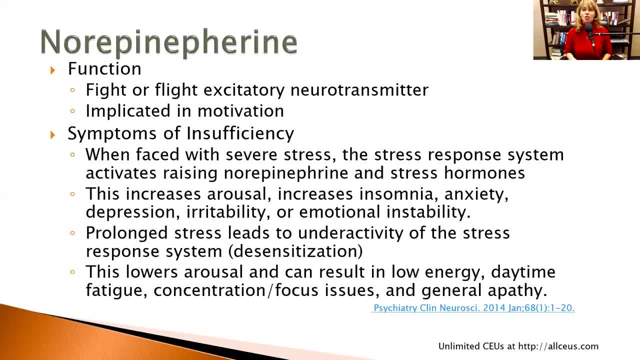 It's implicated in motivation and focus. So norepinephrine goes out. you get that kind of laser focus. When people don't have enough norepinephrine, um then it causes problems with arousal and and a lot of other things. 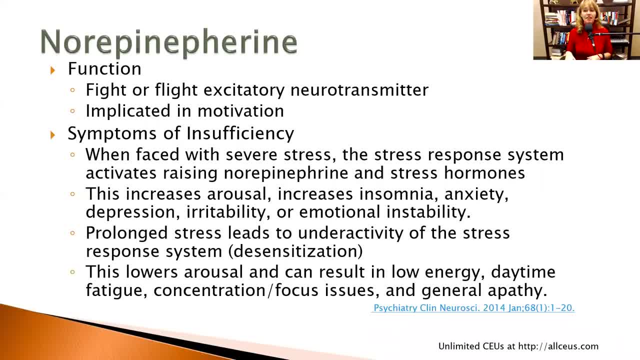 When faced with severe stress, the stress response system, um activates raising norepinephrine as well as other stress hormones, which increases arousal. um increases insomnia. You know you don't want to be sleeping if you're under threat. 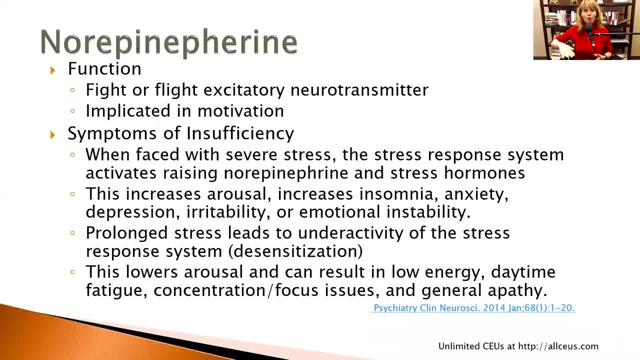 It increases anxiety, irritability, emotional instability and if it goes on for too long, it can also increase depression. So cortisol, if you remember from from other lectures, cortisol causes the body to say: you know, we're going to reduce estrogen right now because we don't have. 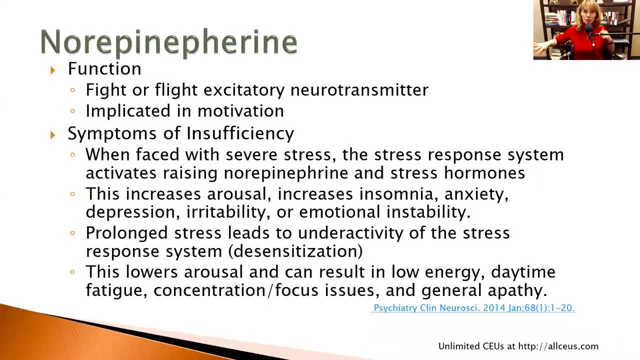 we don't have the need for procreation. there's a threat out here which tells you from the last slide that dopamine levels are going to go down too. Ooh, okay, So, but we also know that serotonin availability is affected by estrogen levels. 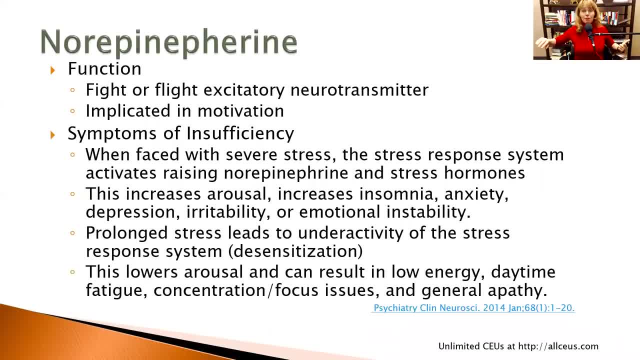 So serotonin is a calming chemical and helps with mood. So dopamine and serotonin go down. when estrogen goes down, Norepinephrine goes up, which increases heart rate and respiration and focus and all kinds of stuff like that. Um, we also know that a lack of um serotonin or less serotonin is going to be implicated. 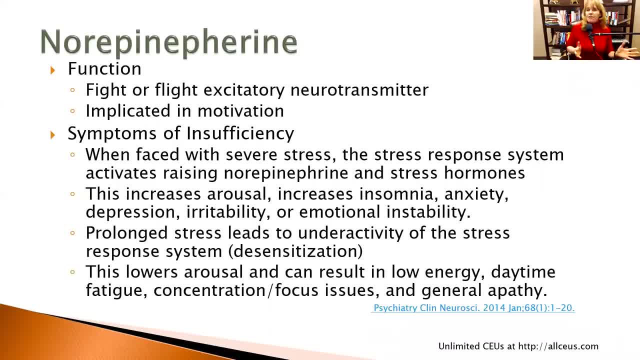 in in sleep problems. So norepinephrine and serotonin are kind of um teeter-totters, You know, when one goes up, the other one tends to go down. Prolonged stress leads to underactivity of the stress response system- desensitization. 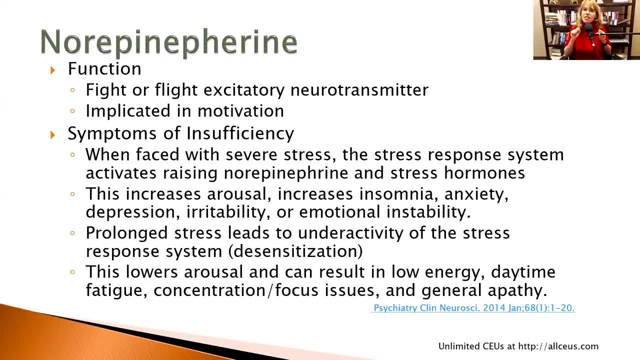 So your brain, over prolonged stress, is going to start saying: you know what? I've only got so much energy and I can't fight or flee from everything right now. I have to conserve it for what's really the most important. So people may not have norepinephrine sent out as much, which is when you start feeling. 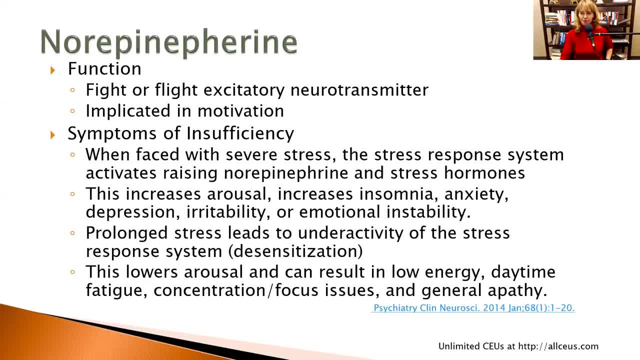 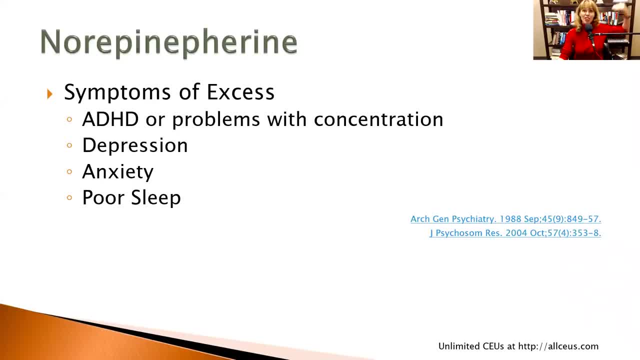 depressed or seeing depressive symptoms, Symptoms of excess norepinephrine, ADHD or problems with concentration. Remember you saw that in dopamine too: Depression: If people are too wild, Round up for too long, they may start experiencing some some depression, anxiety and poor sleep. 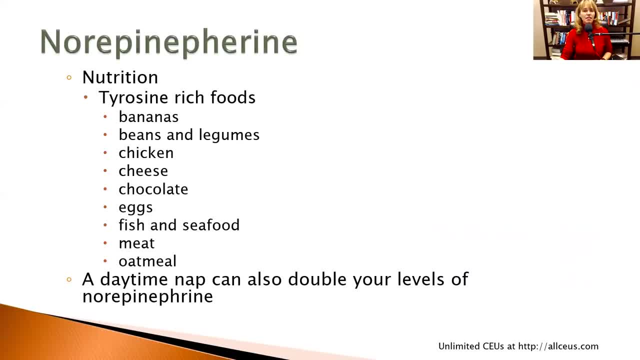 Nutrition- Again tyrosine. rich foods- You want to look at bananas, beans and legumes, chicken cheese, chocolate, eggs, fish and seafood, meat and oatmeal. Um so tyrosine we're. we're seeing repeatedly making sure that people are getting access. 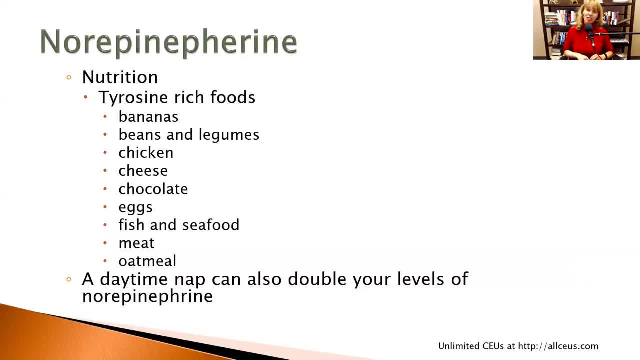 to some of these, And I included. I made sure to include vegetarian options as well, As well as um other options in case people aren't good with eggs, fish or chicken. A daytime nap, they found, can also double your levels of norepinephrine. 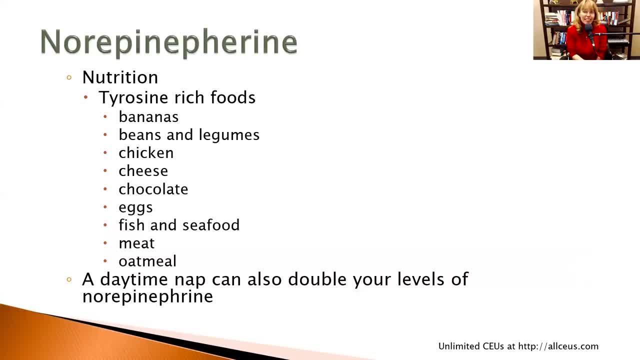 Now, naps should never be well ideally longer than 45 minutes. You don't want people to go into a full REM cycle because that just throws their circadian rhythms completely off. a 20 minute nap where you're resting your eyes- Some people find that that makes them feel a ton better. 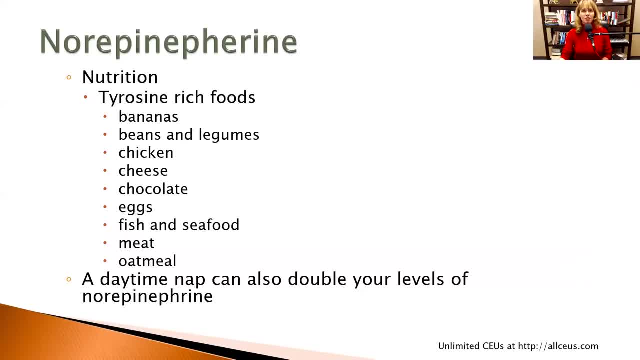 I can't seem to shake it If I lay down for 20 minutes or sit, sit in the easy chair for 20 minutes. I feel groggy afterwards, So people will have to figure out for themselves if that works for them. 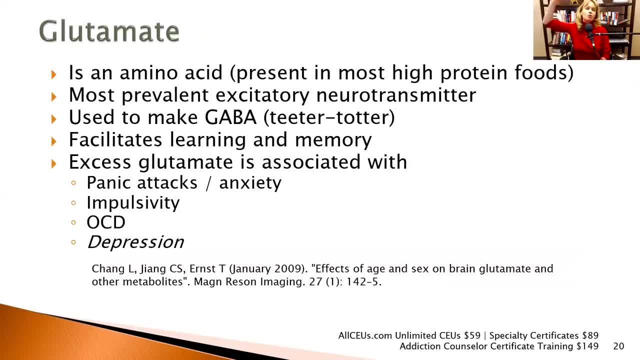 So glutamate is another excitatory neurotransmitter. So dopamine is our pleasure neurotransmitter. It helps keep us motivated. Norepinephrine is our motivation and our fight or flight neurotransmitter. Um glutamate, It's also another excitatory neurotransmitter. 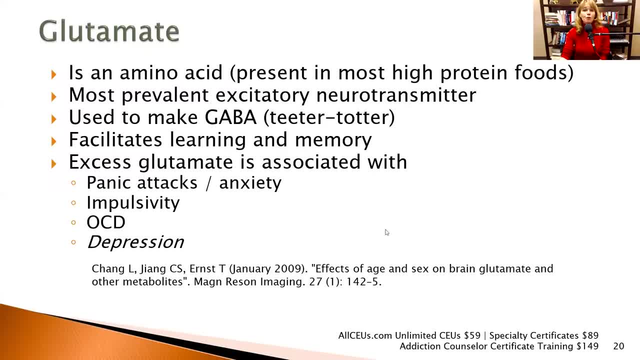 It's going to rev people up. Um, glutamate is actually a, an amino acid which is present in most high protein foods, So you don't even have to go out of your way to find this one. If you're eating protein, you're probably getting it. 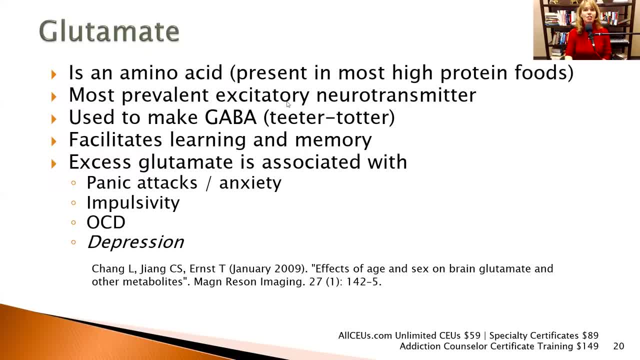 It's the most prevalent excitatory neurotransmitter and it's used to make GABA. The brain breaks down glutamate to make GABA. So if you don't have enough glutamate which revs you up, you're not going to be able to. 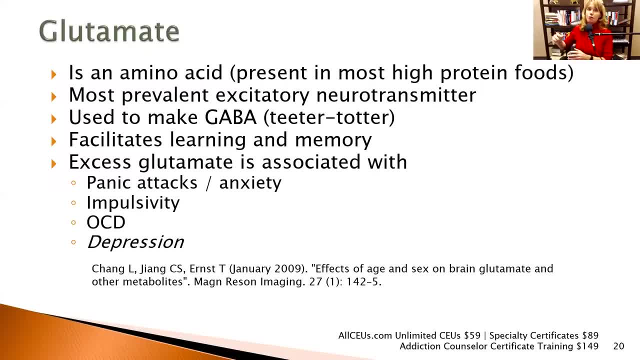 you're likely make enough GABA to calm you down, And GABA is our primary chillax neurotransmitter. It facilitates learning and memory. It keeps us alert. Too much glutamate, though, is associated with panic attacks and anxiety, impulsivity, obsessive. 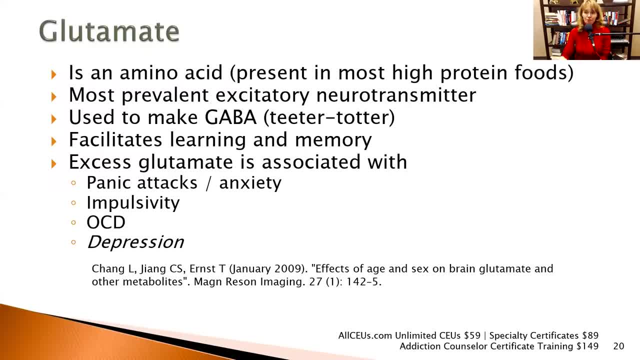 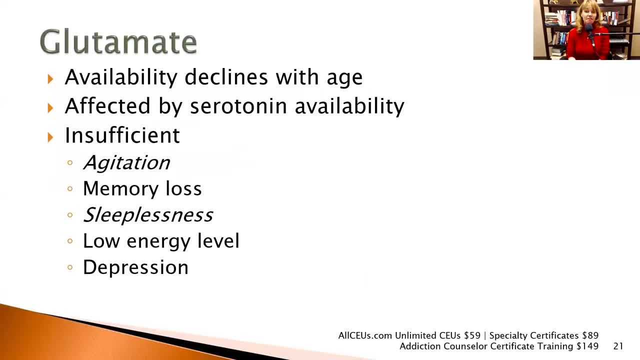 compulsive disorder and sometimes depression. Glutamate availability declines with age And it's affected by stress Serotonin availability. So you know, if there's more serotonin then there's not going to be as much glutamate, and and vice versa. 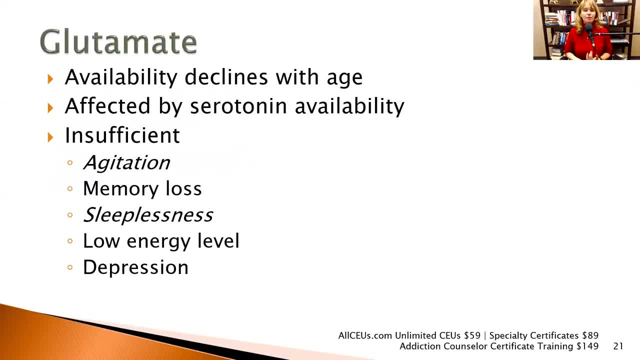 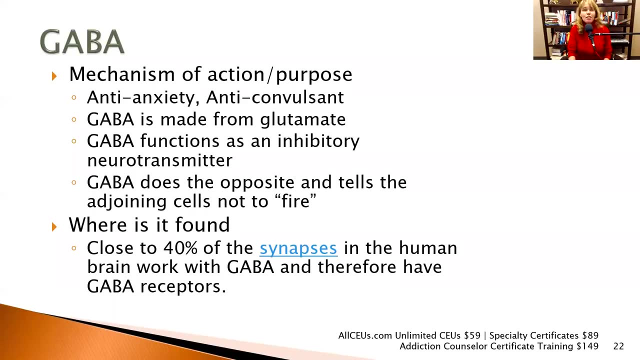 Too little glutamate can lead people to feel agitated, have memory loss, sleepless um, low energy level and depression Glutamate. we don't talk about a lot. We talk more about GABA, and GABA is designed as an anti-anxiety. 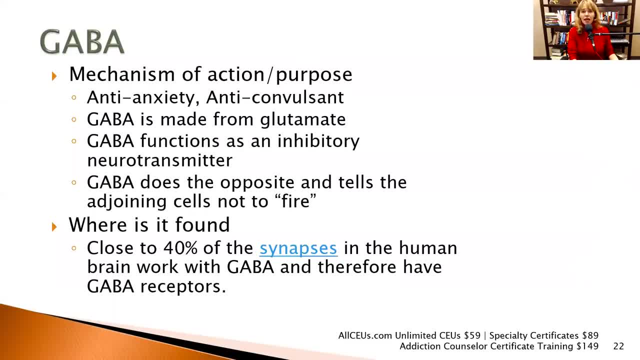 Anti-convulsant sort of neurochemical. It's made from glutamate and functions as an inhibitory neurotransmitter. So it inhibits our functions, It slows our breathing, slows our our heart rate, lowers our blood pressure. You know, it's just a great neurotransmitter. 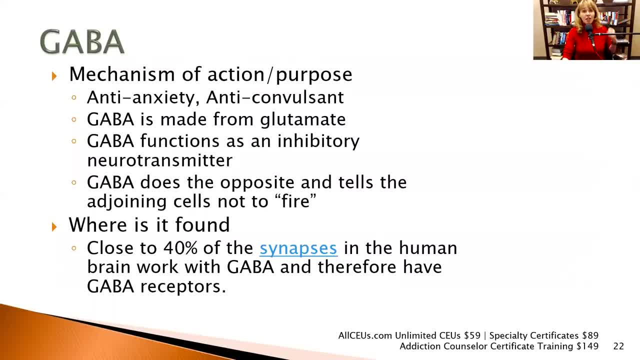 GABA does the opposite of glutamate And instead of telling all the nerves to fire, it says: don't fire, just relax. Close to 40% of the GABA synapses In the human brain work with GABA and therefore have GABA receptors. 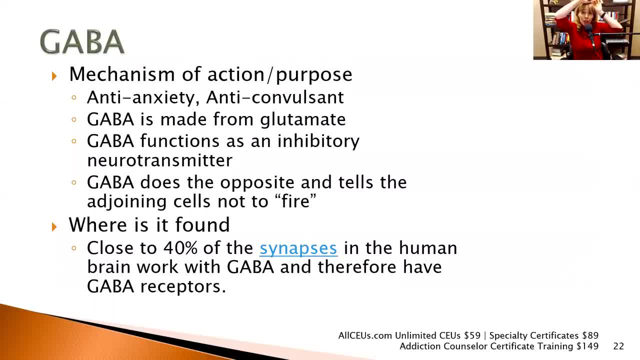 So think about that in your brain- not just in one little part of your brain, but in your brain- close to 40% of the synapses work with GABA. So if you don't have enough GABA, then you could have some significant side effects. 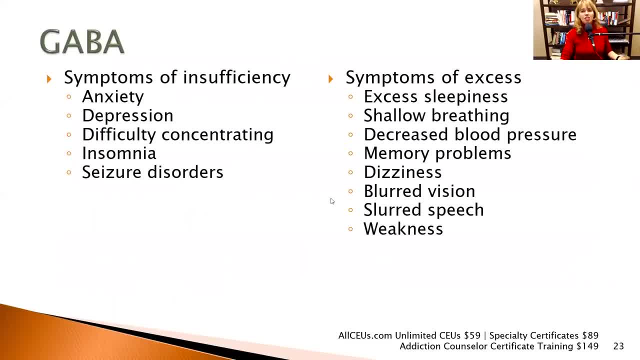 insufficiency, anxiety, depression, difficulty concentrating, insomnia and seizure disorders. Um one of the medications that we'll talk about in a few minutes, Klonopin, is an anticonvulsant and it increases GABA levels. symptoms of excess. 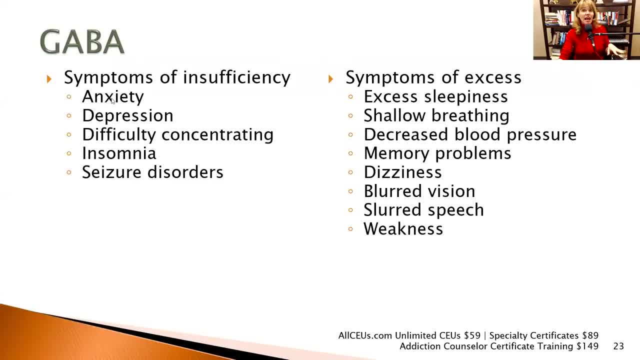 And sometimes you'll see Klonopin prescribed for anxiety as well, you know, because the prescribing physician doesn't like some of the traditional benzos for some reason. Symptoms of excess: excess sleepiness, shallow breathing, decreased blood pressure, memory problems, dizziness, blurred vision, slurred speech and weakness. 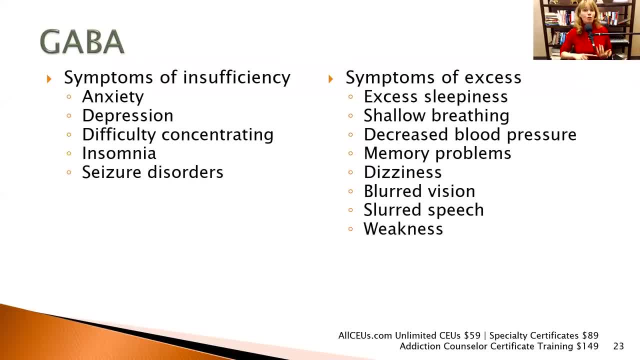 So All the symptoms of what you would see with an opiate- opiate overdose, what you would see with a GABA overdose, what you would see in somebody who's intoxicated. You know, these are the things that we're going to be looking for. 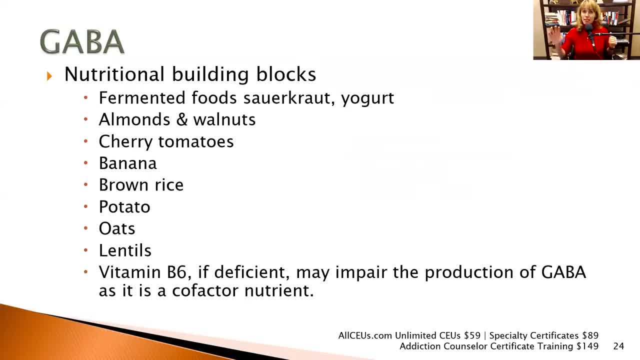 Nutritional building blocks: fermented foods. Now, that's, that's the. this is the only one that nutritional building block is a fermented food: almonds and walnuts, cherry tomatoes- tomatoes with a thicker skin- have more of of what's needed to improve GABA levels. 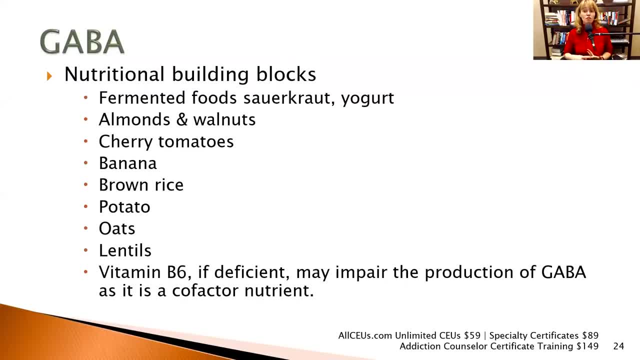 Bananas, again brown rice, again potatoes, oats, lentils. If the person's deficient in vitamin B6, it can impair the production of GABA, Even if they have all the building blocks. it's kind of like trying to build a brick house. 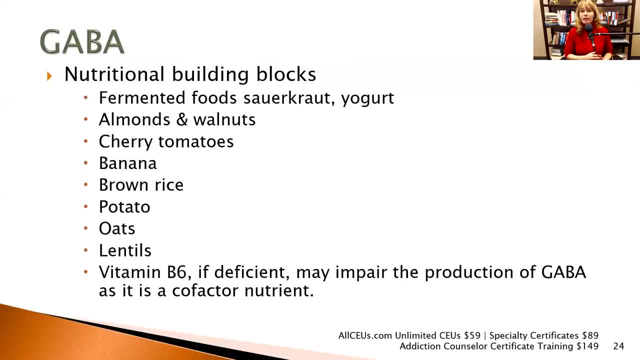 without mortar. so they need to make sure that they're getting enough B6. Most people get enough in their diet and or with a multivitamin, but that's between them. B8 is another one that's really important for GABA. 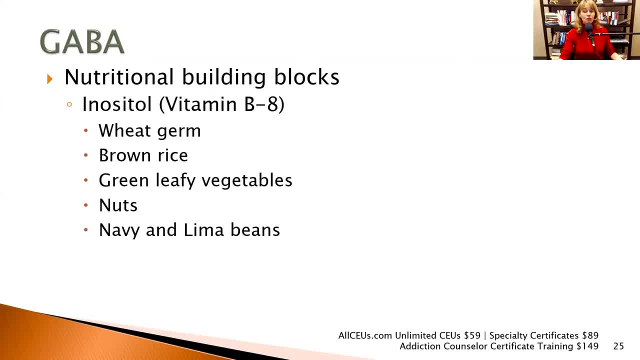 You can find that in wheat germ brown rice, green leafy vegetables, nuts and navy and lima beans specifically. So that may be a little bit harder to get if you don't like brown rice or green leafy vegetables, but it's possible. 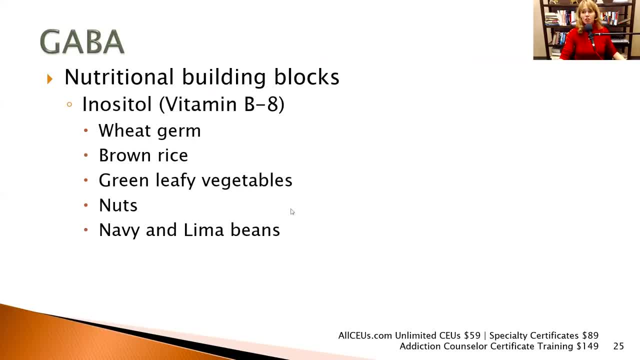 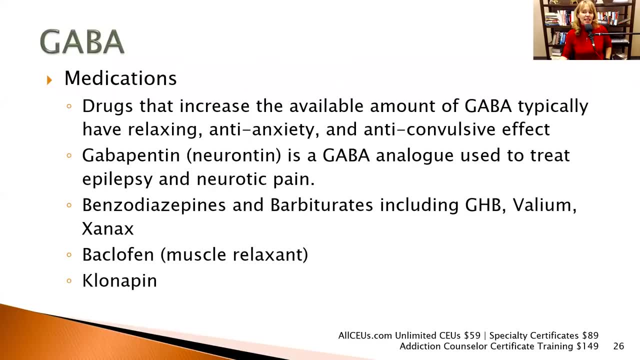 And you know you will find it in some of the better nutritional multivitamins. Medications that increase the available amount of GABA typically have a relaxing, anti-anxiety and anti-convulsive effect. Gabapentin is one of the more common ones that we think of, or Neurontin is a GABA analog. 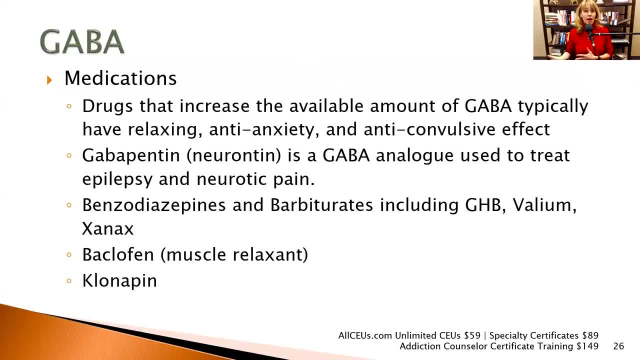 and is used to treat epilepsy and neurotic pain. Benzodiazepines and barbiturates, including GHB, Valium and Xanax, also increase GABA levels. Baclofen, which is a very common drug, is also used to treat epilepsy and neurotic pain. 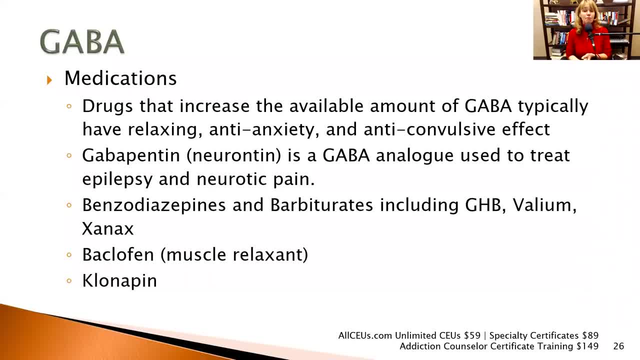 And Klonopin. well, Baclofen is a muscle relaxant. My dog is actually on that right now- She's 14, so- But it's a newer muscle relaxant and painkiller sort of thing. And Klonopin is the anti-convulsant that I told you about before. 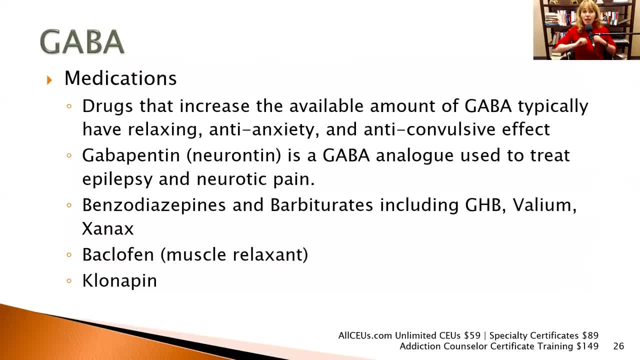 This is not an exhaustive list, but it gives you an idea that we're kind of covering a broad spectrum. If you're working with somebody who has co-occurring issues, the doctors are probably going to steer away from the last three and more towards Neurontin. 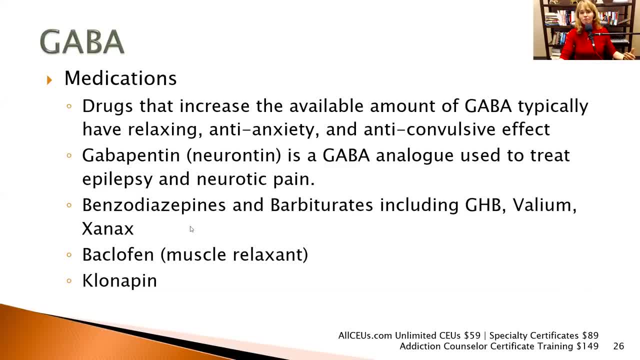 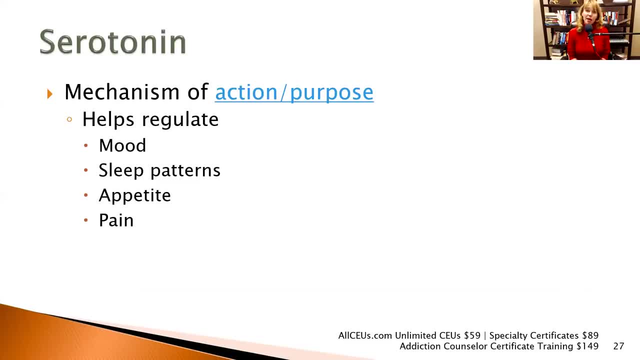 for chronic pain and muscle problems. Now, serotonin, our favorite chemical to talk about, Not mine, but in general. It helps regulate mood, symptoms, mood sleep patterns, appetite and pain, So how you feel, how you sleep, whether you're hungry and if you're in pain. 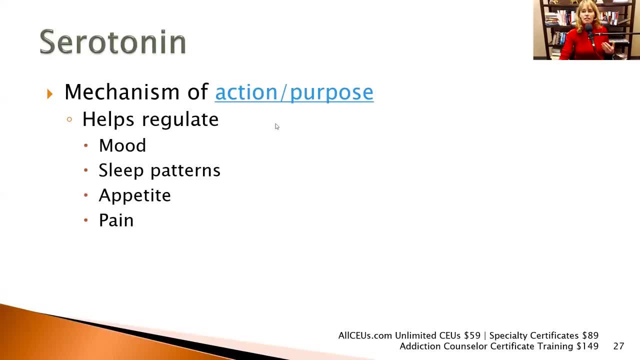 It's a big one And there are a lot of other things that it does. If you go here, let me see if I can get it to come up. Maybe, maybe not, And this is far too small for you to really read right now. 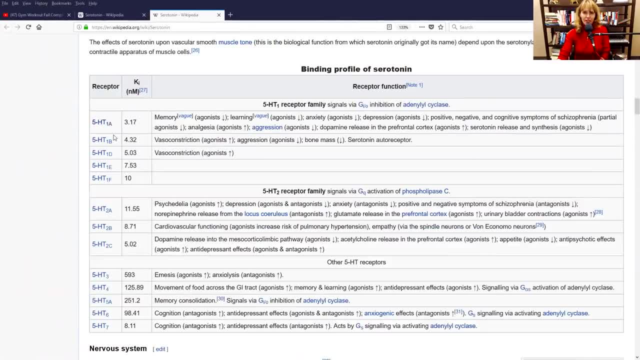 But if you go to this Wikipedia page on serotonin, it talks about all the different serotonin receptors and binding profiles and talks about what it's involved in. Like, 5-HT1A is responsible for dopamine release in the prefrontal cortex, in addition to being 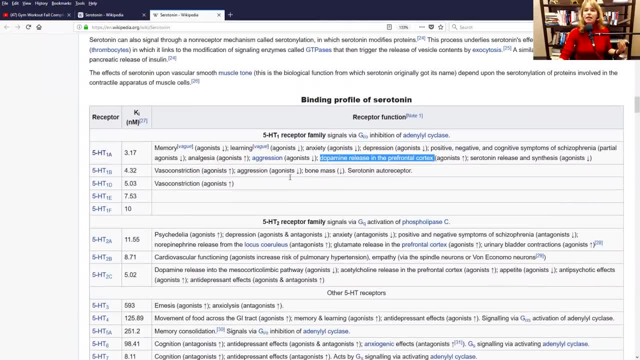 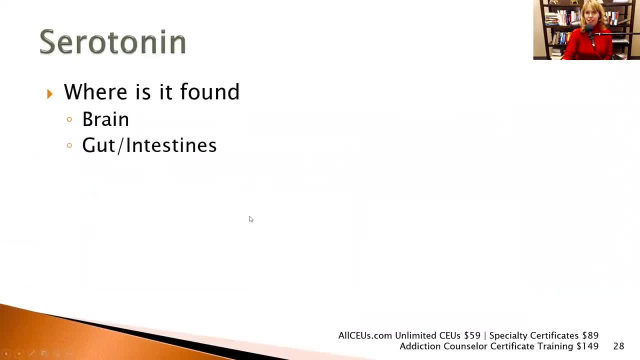 a serotonin receptor. So it gives you an idea about how broadly some of these neurochemicals can affect someone Anyhow. where's it found? It's found in your brain, but 80% of your serotonin is found in your gut and intestines. 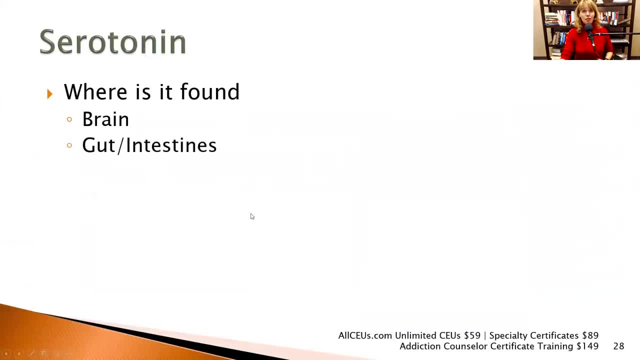 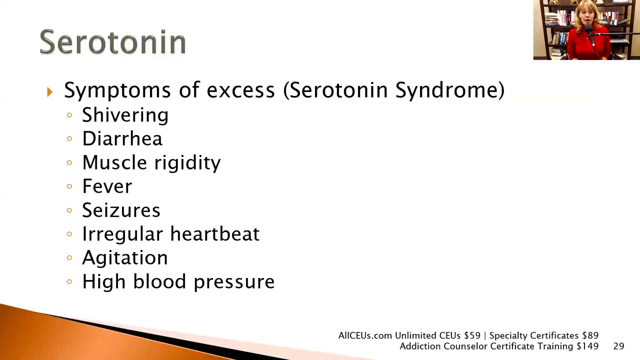 So if you're working with somebody who has gut and intestinal problems that are reducing bioavailability, reducing absorption, you could have some problems here. So brief little talk about serotonin syndrome, because we don't talk about it enough And it's so important. 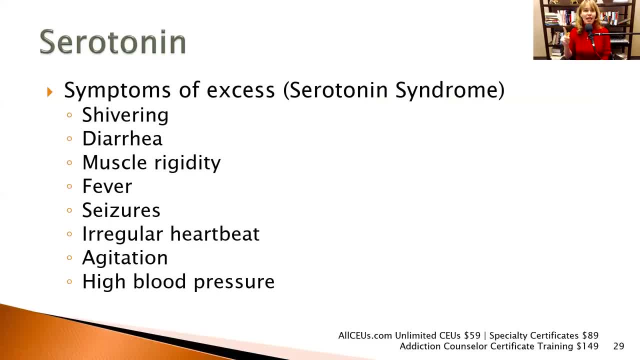 One dose too much One time. It's not something that has to build up over time like most SSRIs do. If you overdose one time, you can develop serotonin syndrome. Now that generally goes away when the offending chemical gets out of your system, but it can. 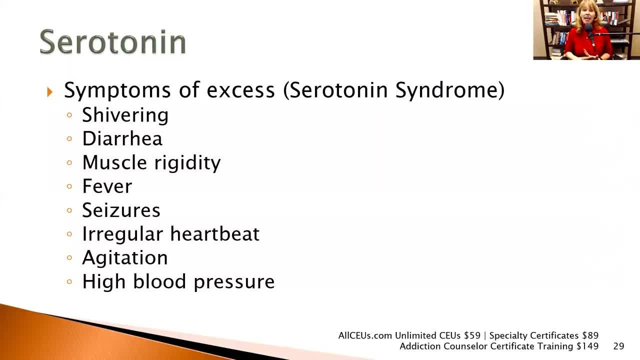 cause shivering, diarrhea, muscle rigidity, fever, high, high fever like 108, plus seizures, irregular heartbeat agitation, high blood pressure, stroke. So it's important to be aware that too much serotonin can be really, really bad. 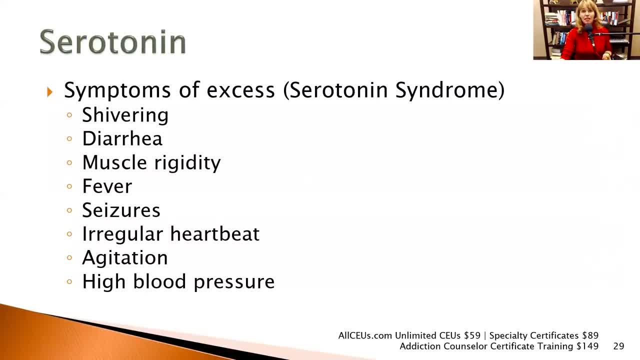 And people who take supplements like 5-HTP can easily get too much serotonin. There are also a lot of other things that you're going to find out in a minute that increase serotonin, that people aren't aware of as being serotonin increasers. So it's really important to educate clients about the side effects so they're more cognizant. 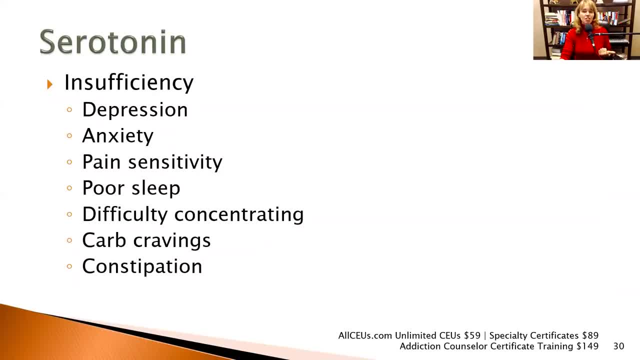 So too little serotonin leads to feelings of depression, anxiety, pain sensitivity. Serotonin is involved in regulating our pain threshold. When our pain threshold is low, we're going to have a lot of pain. When our serotonin is low, our pain threshold is lower. 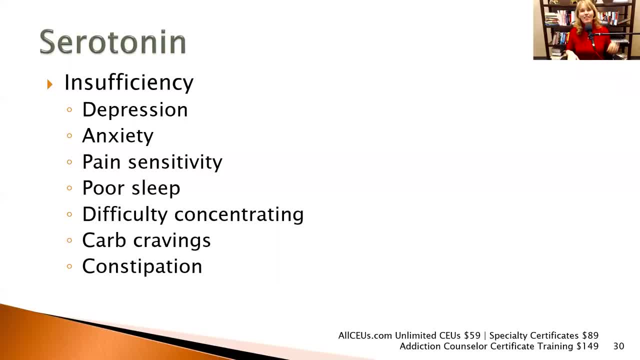 Same thing again with dopamine. When our dopamine is low, our pain threshold is lower, because dopamine helps with pain. Poor sleep because melatonin is made by breaking down serotonin. If somebody doesn't have enough serotonin, they may not be able to get quality sleep. Difficulty concentrating carb cravings. Our body, when we eat high sugar, High carb foods, tends to release serotonin and dopamine. See how these things are so hard to ferret out, especially since we can't really experiment on the human brain. Anyhow, carb cravings are common in people who have, or we believe in people who have. 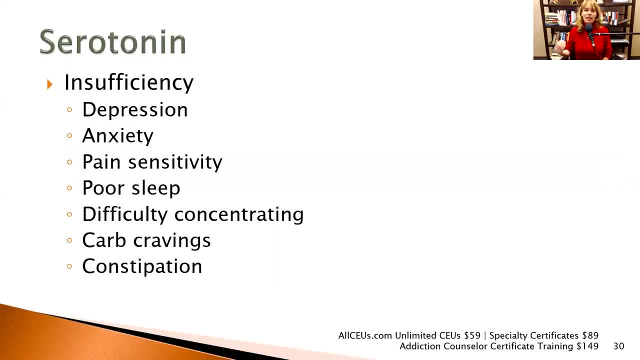 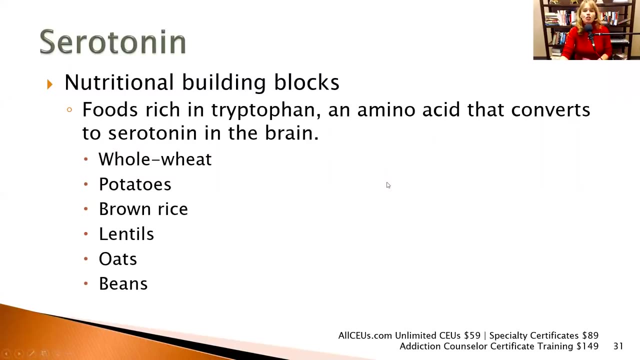 low serotonin And constipation. Serotonin keeps everything moving. If somebody has hypothyroid or low serotonin, they could have constipation caused by either one of those. among other things, Nutritional building blocks Are foods rich in tryptophan. 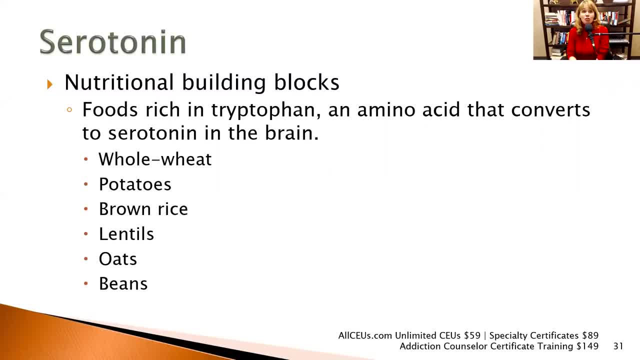 The body cannot make tryptophan, so you have to get tryptophan from what you eat: Whole wheat, potatoes, brown rice, lentils, oats and beans. I feel like a broken record when I read this, So hopefully your clients are willing. 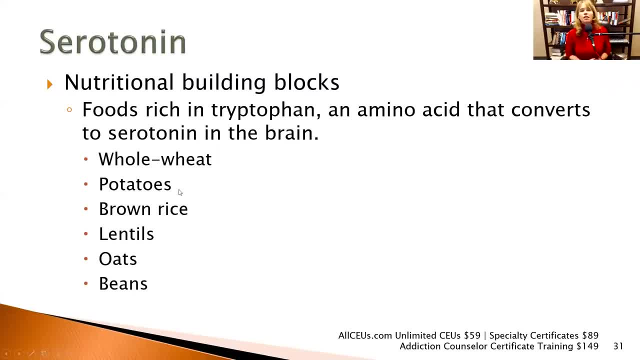 So look at something in here And if they don't like these options- obviously they're working with their nutritionist- They can go online and Google- I believe it's world's healthiest foods- and find out which foods are high in tryptophan and find something that suits their fancy a little bit better. I just listed the top ones. Medications and supplements that increase serotonin. Selective serotonin reuptake inhibitors. Obviously, we know that's the first line For a lot of people. when they're depressed, doctors give them SSRIs. your Paxil Prozac. 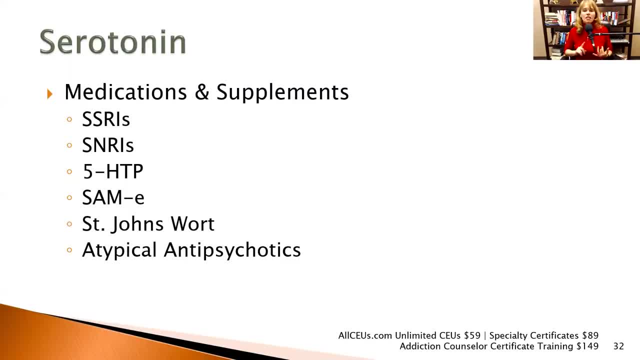 Zoloft, Lexapro, yada yada. Selective norepinephrine reuptake inhibitors also make the serotonin more available. They prevent the reuptake of serotonin as well as norepinephrine 5-HTP increases serotonin. 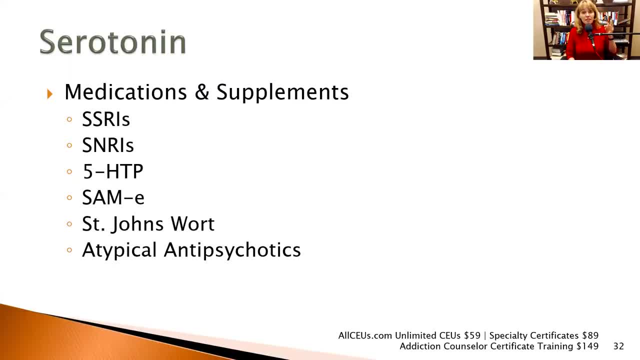 SAMe, St John's wort, The last three, 5-HTP, SAMe and St John's wort. people can buy over-the-counter, which can be really scary because they can accidentally get too much. Atypical antipsychotics have been used in people for whom the first line SSRIs and 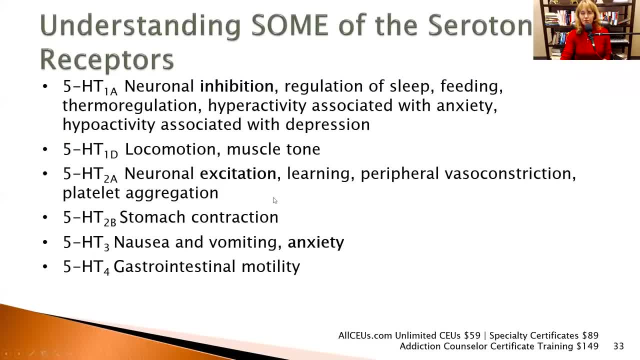 SNRIs didn't work. Some of the serotonin receptors are responsible for sleep regulation, feeding thermoregulation. so if people are getting cold a lot or too hot, Hyperactivity, hypoactivity, locomotion, muscle tone, learning, peripheral vasoconstriction. 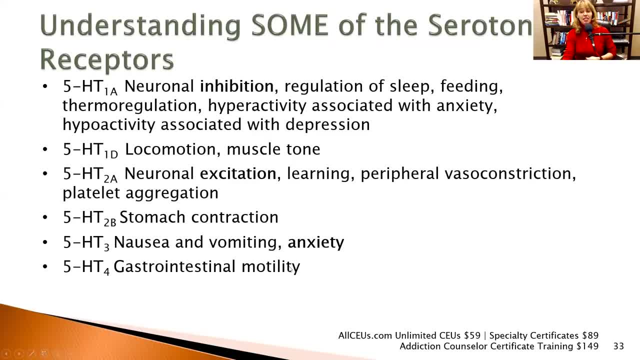 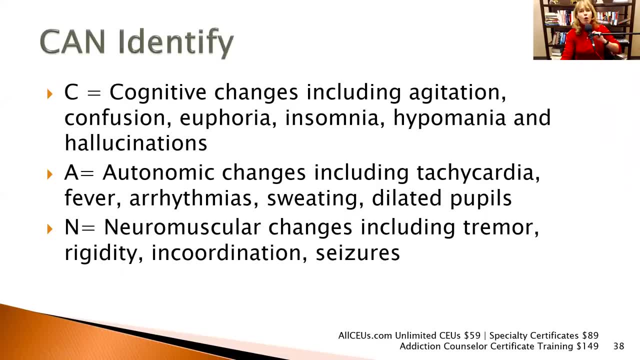 stomach contraction, nausea and vomiting, and gastrointestinal motility, And you're like, okay, why do I care? Because, oops, where did it go When we- I'm going to jump around a little- When somebody has serotonin syndrome, there are three things that we're going to look. 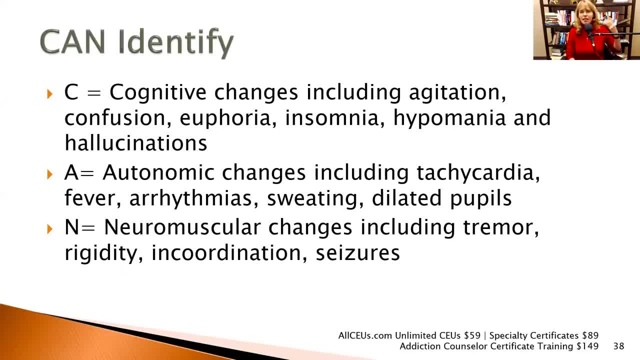 for: And it's the acronym. What's the acronym? Or mnemonic CAN, Cognitive changes, including agitation, confusion, euphoria, insomnia, hypomania and hallucinations. A stands for autonomic changes, including racing heart, fever, arrhythmias, which is 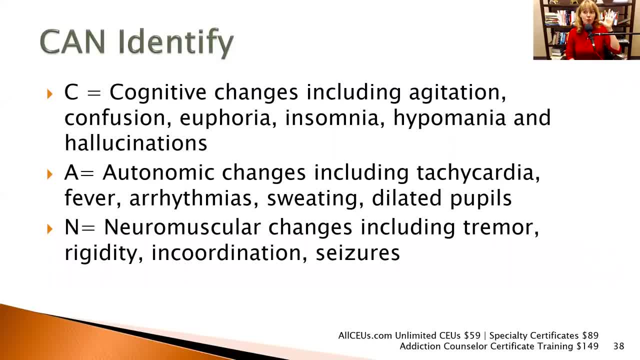 an irregular heartbeat, sweating and dilated pupils, And N stands for neuromuscular changes, including tremor rigidity, incoordination and seizures. If you see this, it's a medical emergency. Just don't even think about. well, is it dopamine? 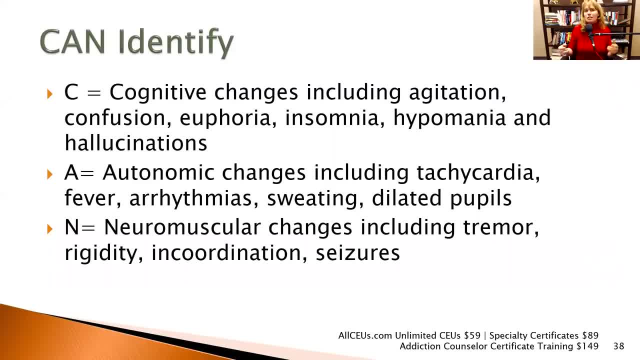 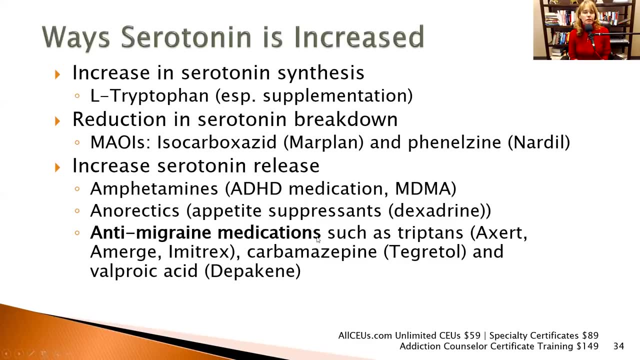 Is it serotonin? Is it alcohol? What's going on? If you see these, it's likely that there's a problem and they need to be evaluated by a medical professional ASAP. So how do we increase serotonin? Because this is another thing that trips people up. 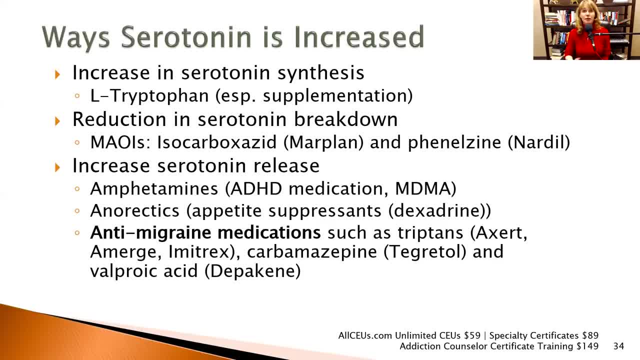 They think the only way you can do it is by taking a psychotropic drug. You can increase serotonin synthesis, like taking an ABV or opioids or something like that, like taking L-tryptophan through supplementation, So you can get pure L-tryptophan and you can ingest it. 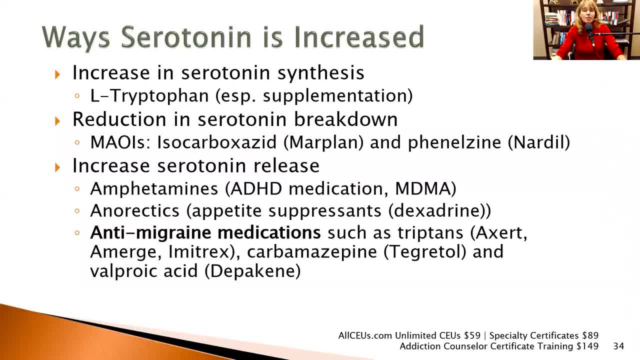 The likelihood of causing serotonin syndrome from supplements, from amino acid supplements. it's really pretty low, but it's not something I'd want to play with. Reduction in serotonin breakdown. So instead of increasing the serotonin available, we just keep what's there from being broken down. 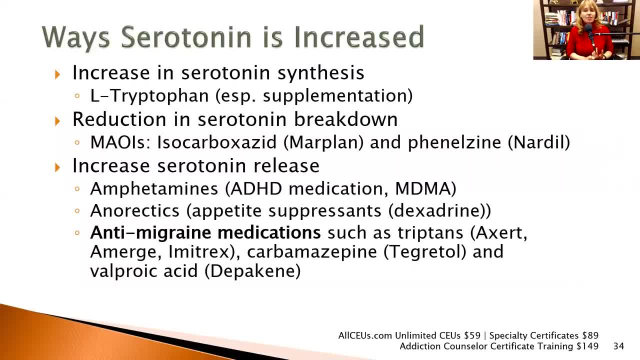 Your MAOIs do that. We can increase serotonin release. Things that cause that include your amphetamines, ADHD medications, MDMA, anorectics, any of your appetite suppressants, weight loss drugs like dexedrine, Anti-migraine medications- and this is a big one- such as triptans. 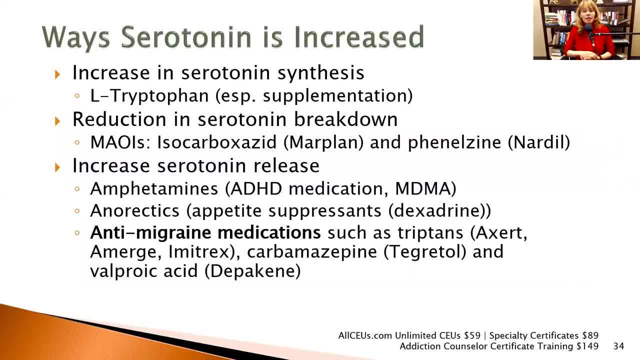 Anti-migraine medications prevent the serotonin or increase the release of serotonin. And if somebody is also taking a selective serotonin reuptake and they're not taking the serotonin, they're not taking the serotonin- Then they're giving themselves a double whammy. 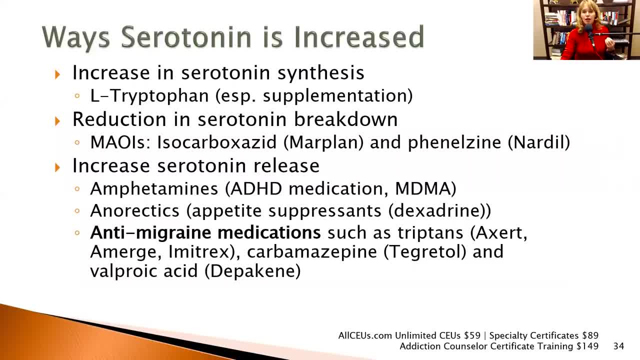 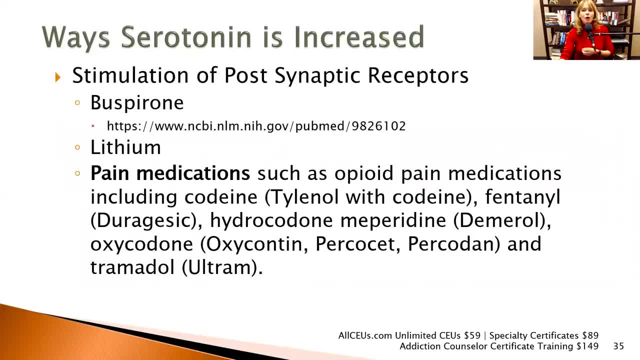 So they need to make sure that they're aware, and their doctor's aware, if they're on an SSRI and prescribed anti-migraine medication. We can also stimulate postsynaptic receptors. Buspirone does this, So it increases dopamine and it can increase serotonin. 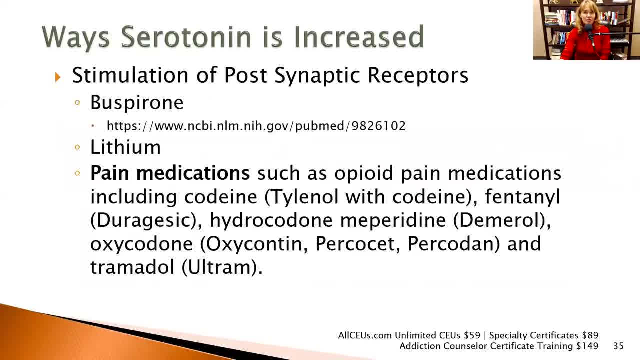 Lithium and pain medications. So again, you wouldn't have thought opiates increase serotonin, but they do, So it's important. And Tylenol with codeine, fentanyl, hydrocodone, oxycodone and tramadol. 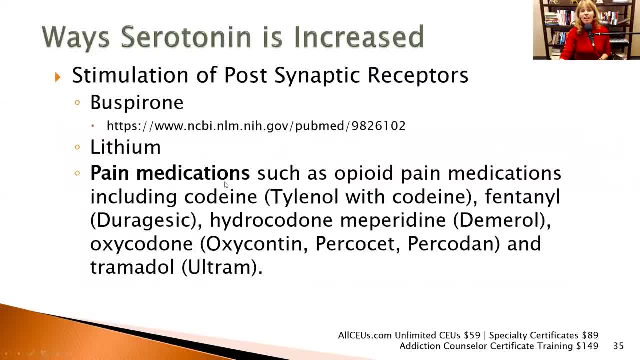 are some of your more common pain medications. If you have a client who goes in for surgery, even oral surgery, outpatient surgery- and they're taking an SSRI or they're taking 5-HTP as a supplement, make sure they know that the pain medications that they may be prescribed. 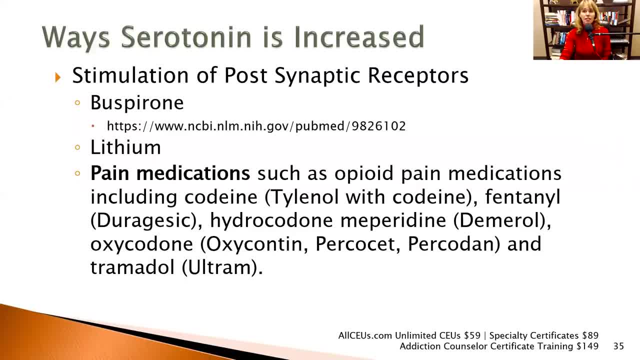 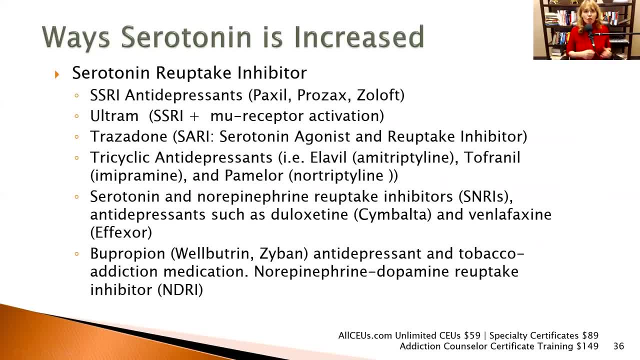 could also increase serotonin and what to look for in terms of serotonin And serotonin reuptake inhibitors? The last one: we have it, we keep it from being broken down and then we keep it in a synapse longer. Your typical SSRIs. 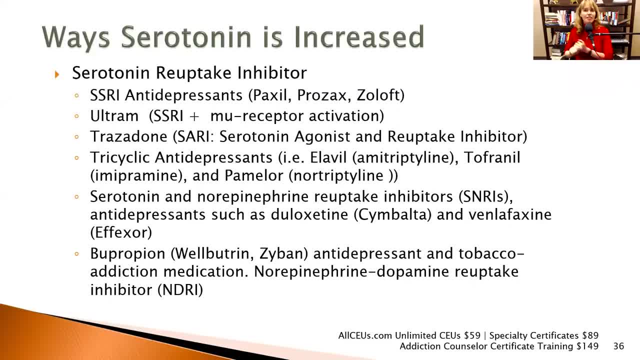 Ultram is also a painkiller as well as an SSRI, So that can be a double whammy. Trazodone is a serotonin agonist and reuptake inhibitor. Okay, So it increases serotonin and it prevents reuptake, which makes it more available. 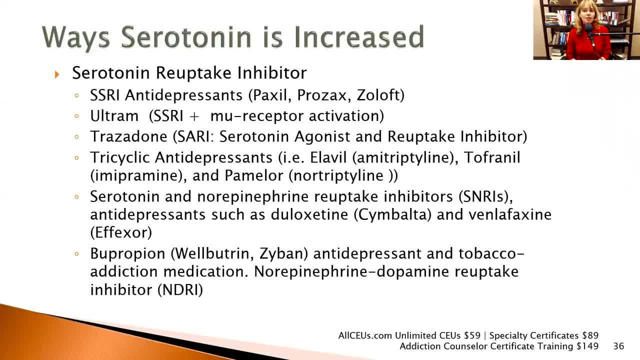 Your tricyclic antidepressants, your serotonin and norepinephrine reuptake inhibitors, and bupropion, which is Welbutrin or Zyban, is also a norepinephrine dopamine reuptake inhibitor. All of these can increase serotonin, as well as norepinephrine and dopamine. for the last one, 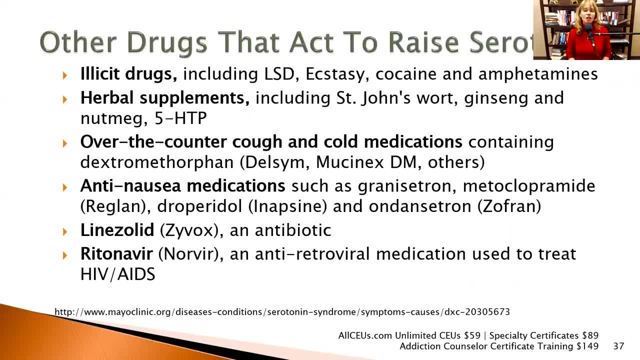 Other drugs that act to raise serotonin. Illicit drugs, including LSD, ecstasy, cocaine and amphetamines, Herbal supplements, St John's wort, ginseng, nutmeg- are added to the list of 5-HTP and SAMe. 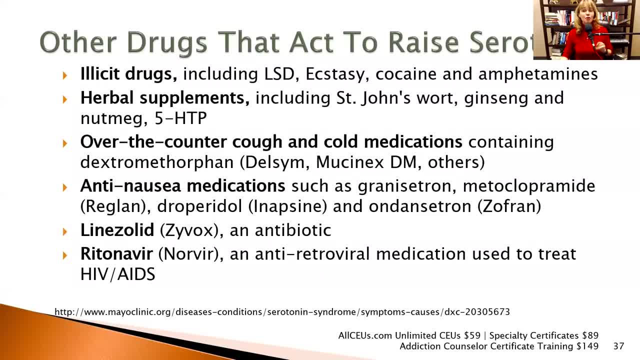 Over-the-counter cough and cold medications containing dextromethorphan- Delsim, Mucinex, DM and others. Some of the youth today are using dextromethorphan Rectally in order to get high off of it. 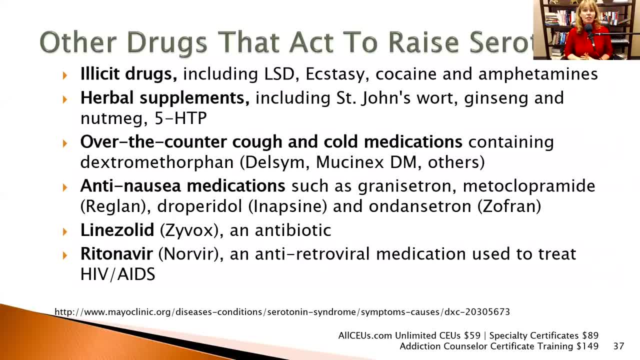 And so knowing that they can actually cause serotonin syndrome by overdosing on dextromethorphan, there's a really fine line between getting high and causing yourself to go into serotonin syndrome. Worth being aware of Anti-nausea medications such as metoclopramide, which is Reglan, and Zofran. 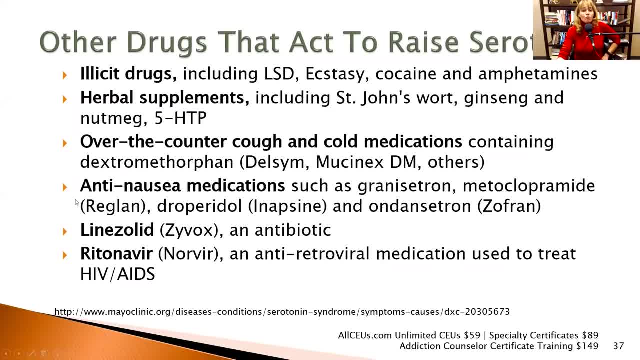 I can read that one. So again you see Reglan, which we talked about under, dopamine also may increase serotonin. So it's important to be aware that if somebody is on an SSRI or you know, a dopamine agonist, 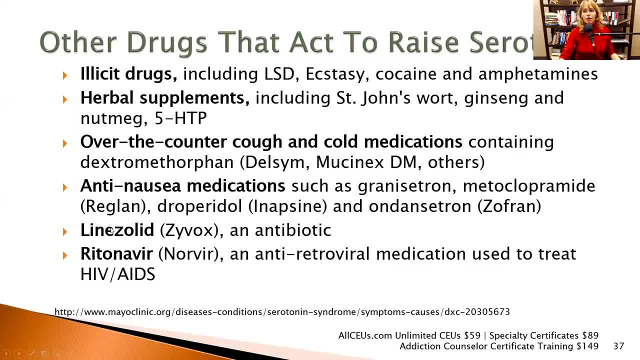 it's important that they also be aware that Reglan is possibly contraindicated. Zovox is an antibiotic. Who knew an antibiotic could increase dopamine, Or not dopamine, but serotonin? It's not one that I've ever seen prescribed, but obviously it is. 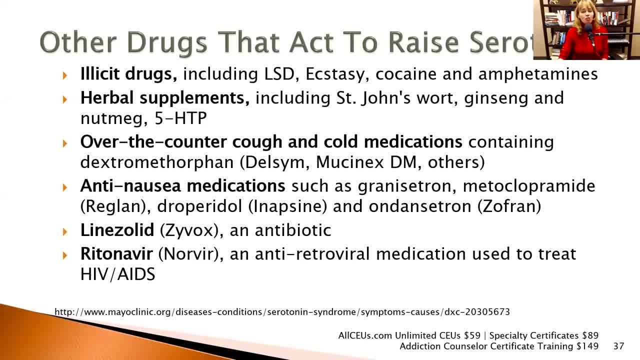 And Norvir, which is an antiretroviral medication used to treat HIV and AIDS, And I have seen this one prescribed a lot. Doctors need to be aware, Clients need to be aware, Because not all doctors are aware of all of these things that increase serotonin. 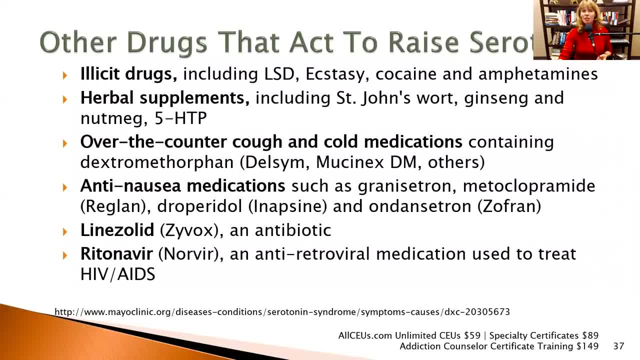 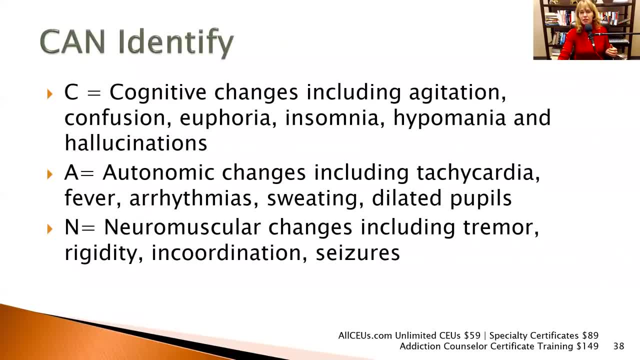 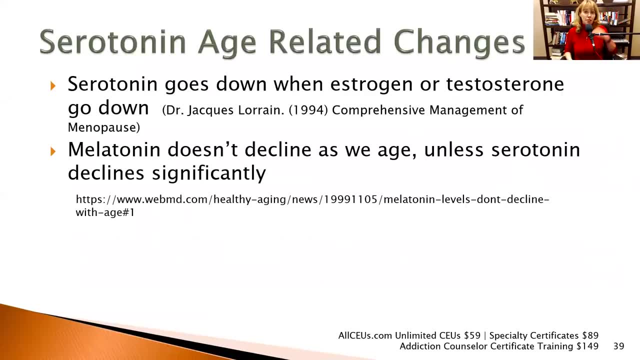 And unfortunately, right now the studies still show that only about 60% of doctors are really aware of serotonin syndrome And think to look for it. Serotonin does change with age. It goes down when estrogen or testosterone go down. So you know, guys, you don't get a pass on this one. 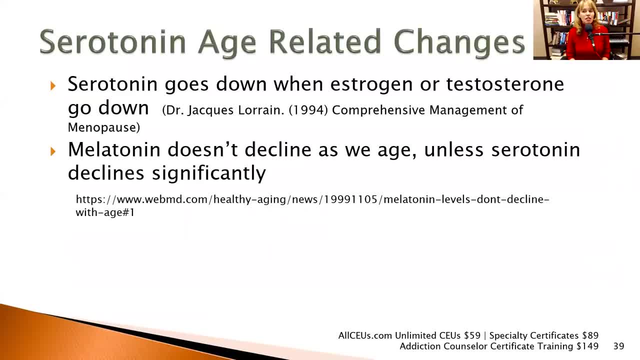 Melatonin, however, doesn't seem to decline as we age, unless serotonin declines significantly. So, generally, the amount of serotonin we need to make enough melatonin to sleep through the night. even as serotonin goes down, it doesn't go down enough to affect our melatonin. 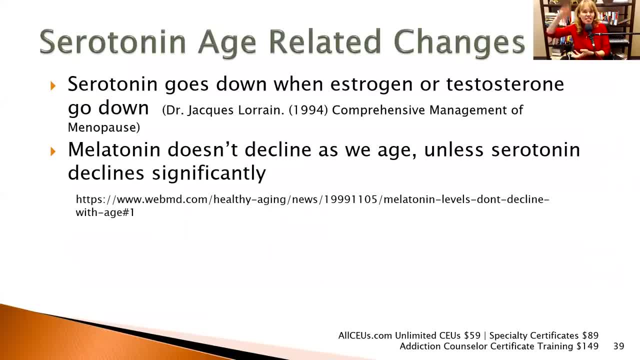 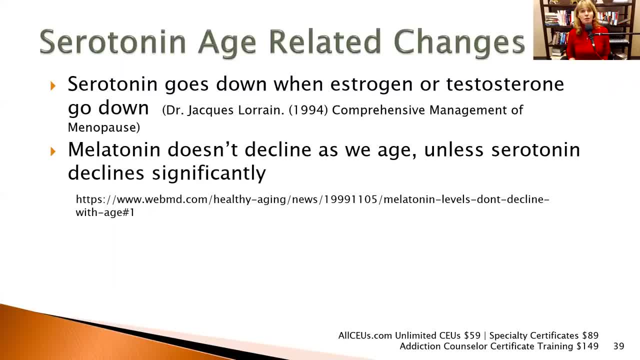 production. Some people find that melatonin supplementation does help them sleep. That's something to consider with their doctor. There are new studies out as an aside that long-term taking of sleep aids- what am I thinking of? like Benadryl, antihistamines- can increase risk of. 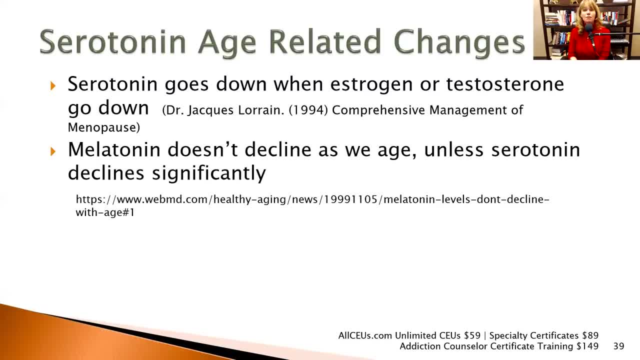 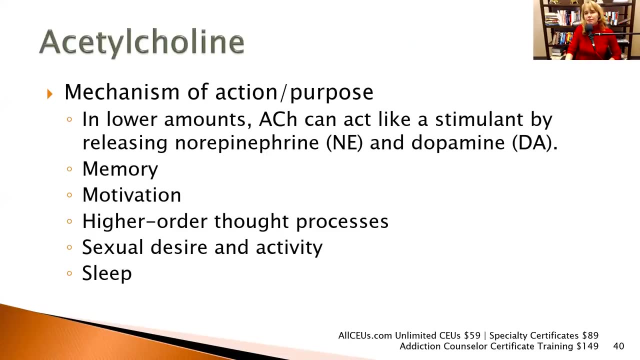 dementia. So people are advised not to use sleep aids for long periods of time and they need to talk with their doctor about other options and, you know, try to figure out why they're having difficulty sleeping. Acetylcholine: See, I told you we would whip through these things. The mechanism. 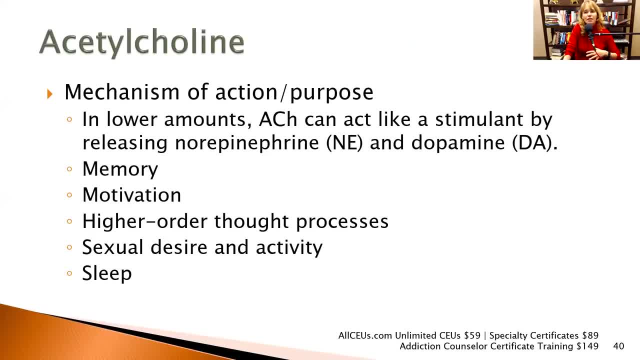 of action. In lower amounts, acetylcholine can act like a stimulant by releasing norepinephrine and dopamine. It also enhances memory, motivation, higher order thought processes, sexual desire and activity and sleep- One of the things well, 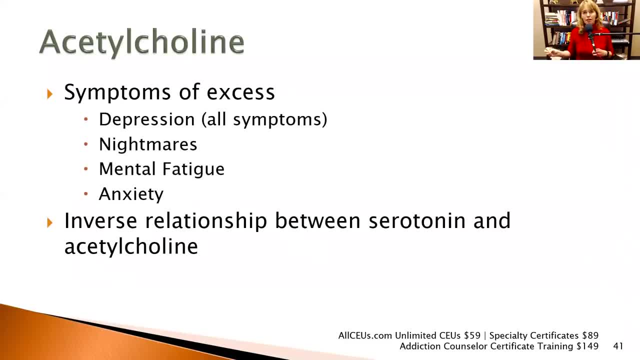 I don't want to get ahead of myself. If there's too much acetylcholine, the person may have all the symptoms of depression, nightmares, mental fatigue and anxiety. There's an inverse relationship between serotonin and acetylcholine, So as serotonin goes down, acetylcholine goes up. 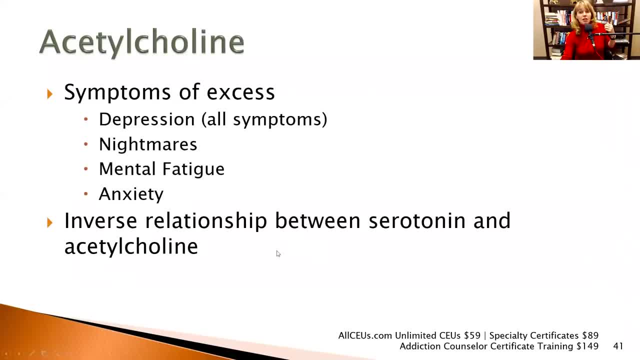 So if somebody doesn't have enough serotonin, then they might start experiencing depression, nightmares, mental fatigue and anxiety. If they take an SSRI increases their serotonin. theoretically their acetylcholine is going to go down, So then they'll start feeling. 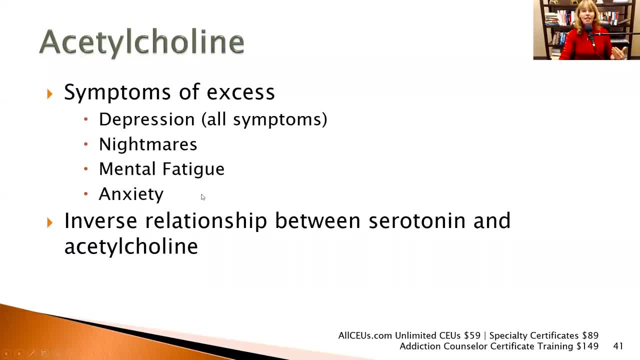 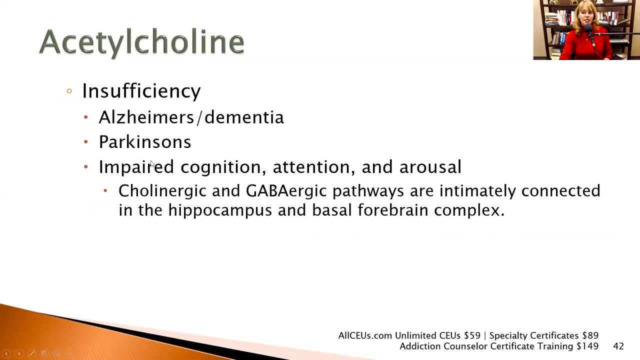 better. Whether it works that way for your particular client is really going to depend on which neurochemicals are out of balance for them. Too little acetylcholine leads to symptoms of Alzheimer's and dementia, Parkinson's, impaired cognition, attention and arousal. So this is another one of our sort of 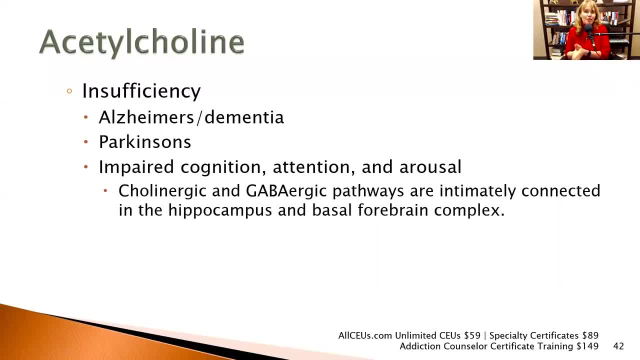 it's not. they call it a modulating neurochemical. It's not necessarily excitatory, but it's not necessarily inhibitory. But we do see, when there's not enough acetylcholine that people start experiencing, you know, tremors, cognitive problems and difficulty with attention. 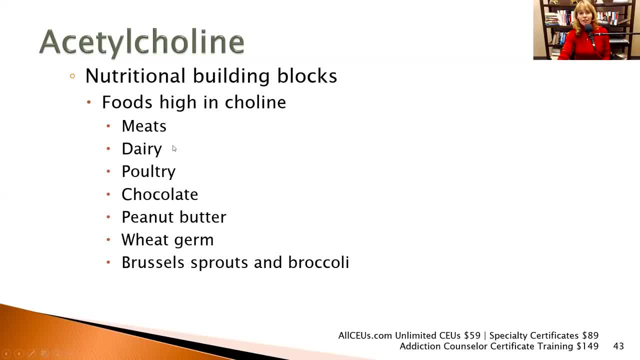 Nutritional building blocks, Foods high in choline, That's easy to remember: Meats, dairy poultry, chocolate, peanut butter, wheat germ, Brussels sprouts and broccoli. Now, I don't know about you, I've never developed a. 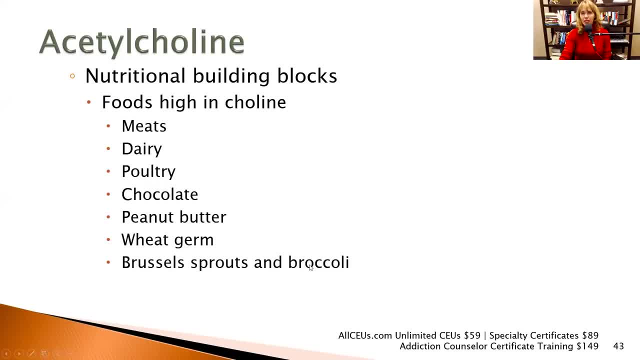 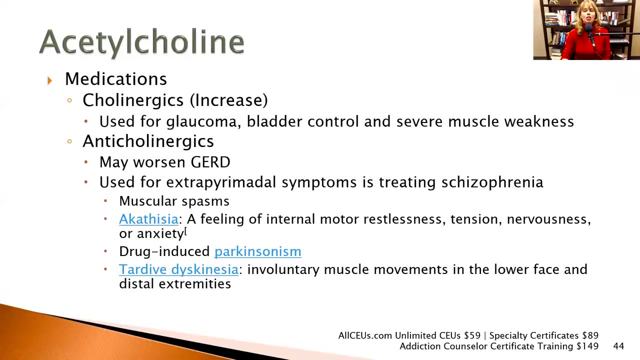 taste for Brussels sprouts, but broccoli I can work in. Wheat germ is pretty easy to get most people to consider Chocolate, poultry and dairy. There's also a lot of acetylcholine in eggs. So the medication Medications. Cholinergic medications are used for glaucoma, bladder control and severe muscle. 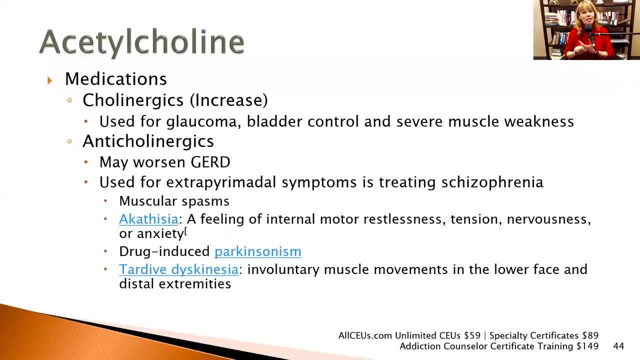 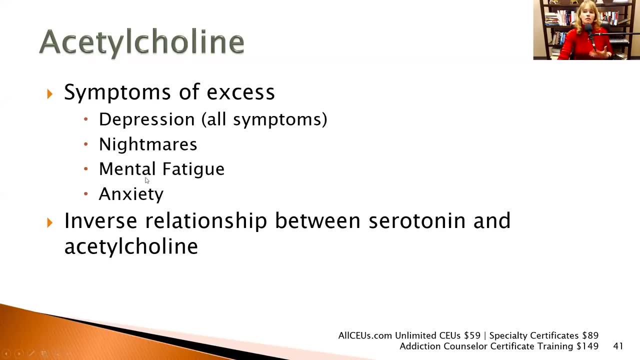 weakness. So we see this sometimes in especially more so in older adults than in younger adults. So they may be on medications that increase their acetylcholine, So we could go back here to symptoms of excess If they start having anxiety, mental fatigue, depression or nightmares. 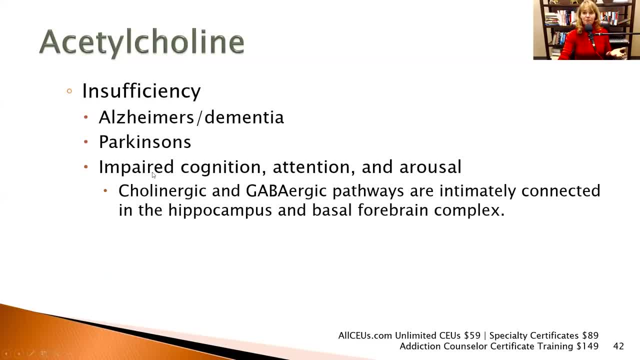 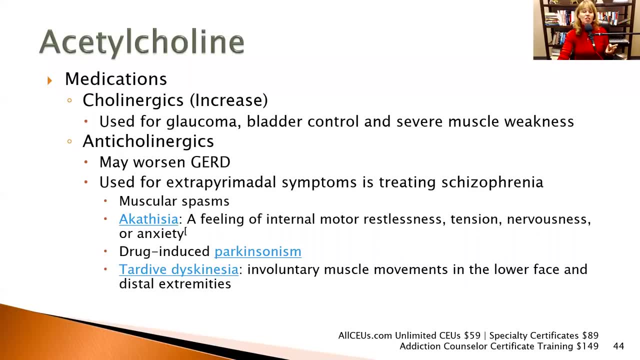 um, that may be a side effect to the medication. They need to talk with their doctor. Anticholinergenics- cholinergics, sorry, may worsen gastroesophageal reflux disease. So if they're taking it and their 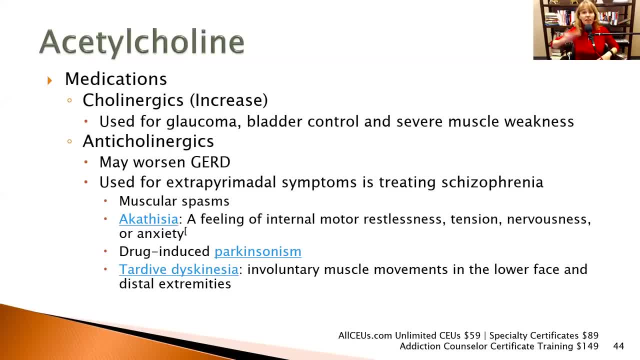 acetylcholine is reduced, they may have more reflux problems. These medications, anticholinergics, are used for extra-pyramidal symptoms with schizophrenia, such as muscle spasms, a feeling of motor restlessness, tension, nervousness. 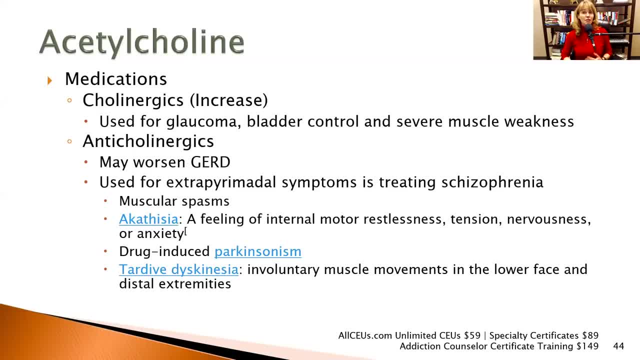 or anxiety, drug-induced Parkinsonianism, trembling, shaking, loss of muscle control and tardive dyskinesia, which is the involuntary muscle movements in the lower face and distal extremities. So if people are having side effects, uh, from some of their, and it's generally. 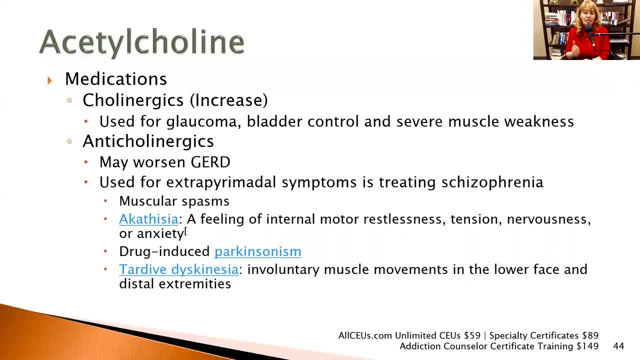 your, your, uh, antipsychotic medications then well, obviously with schizophrenia. then acetylcholine. uh, maybe they may be getting too much acetylcholine, So the doctor may prescribe medication to reduce that too. Now, depending on the person you know, they may not be able. 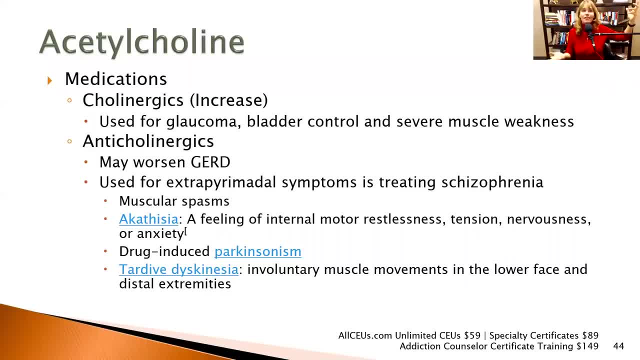 to come off, whatever antipsychotic they're on, So we have to medicate the side effects. That is probably going to produce some side effects, which is how people end up on like seven different medications, Medications that are anticholinergic- atropine, benzatropine. 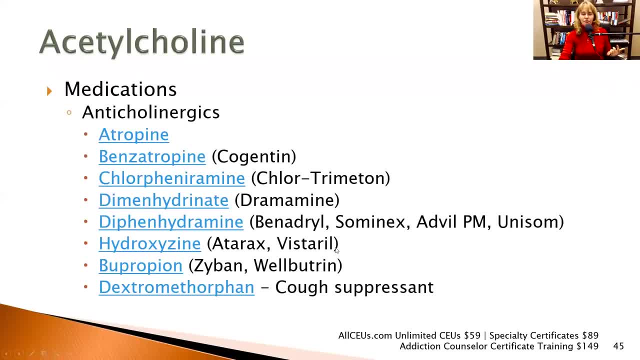 and I have the um brand names over here So you may have seen them on on client charts: Um chlorpheneramine, which is uh. chlorotrimetone Demenhydrinate, which is dramamine, It, you know, seasick. 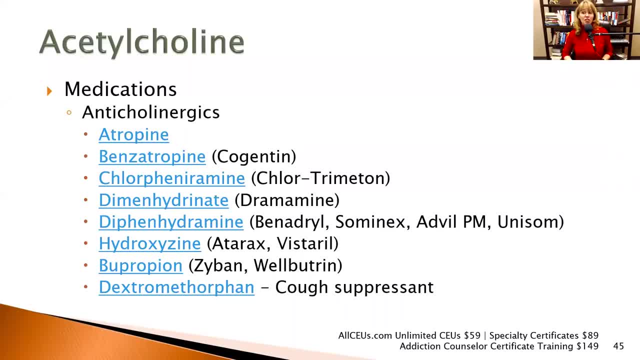 medication, Diphenhydramine, which is Benadryl, Sominex, all your sleep aids, Hydroxazine, bupropion and dextromethorphan are all anticholinergic. So again, if they're taking a prescription drug for, for something um, for for a neurotransmitter. 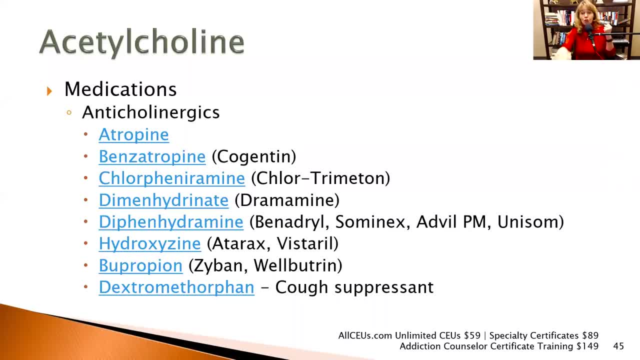 and they start taking any of these over-the-counter ones or prescribed drugs um. it's important that they're aware of the interaction, because people um will not think twice about taking a Benadryl if their allergies are acting up, or taking dramamine if they're getting ready. to go on a flight and they can have really unexpected effects. So, um, if they're taking a dextromethorphan, you know I haven't seen any reports that have indicated that, when taken as prescribed, you know if you've got a cold that it interacts negatively with. 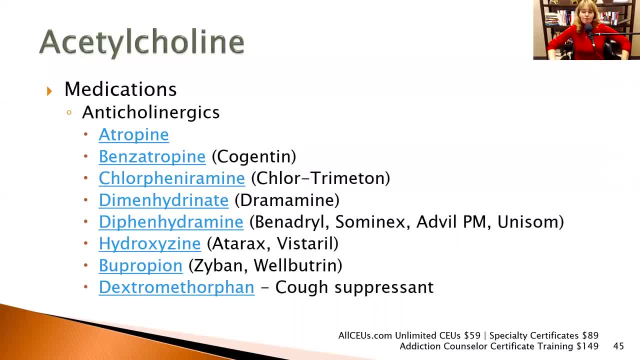 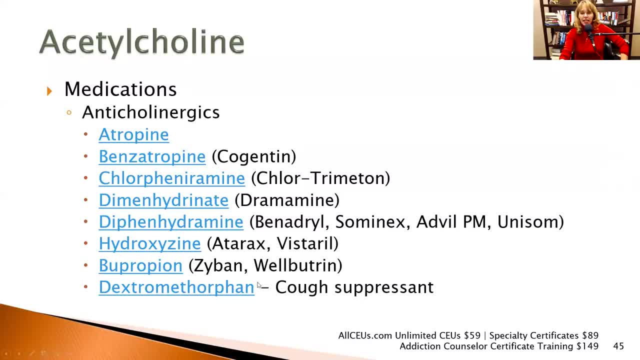 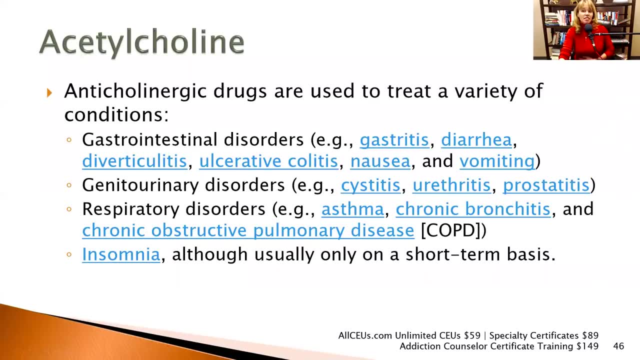 and quintuple the amount of of medication that they're supposed to take. Anticholinergic drugs are used to treat a variety of conditions, including gastrointestinal disorders, which you know. think about your clients, what they have- genitourinary disorders, respiratory. 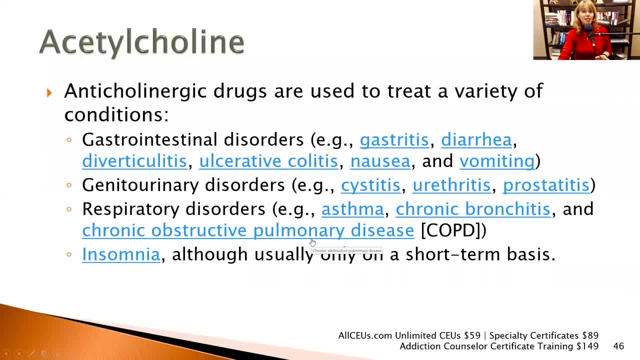 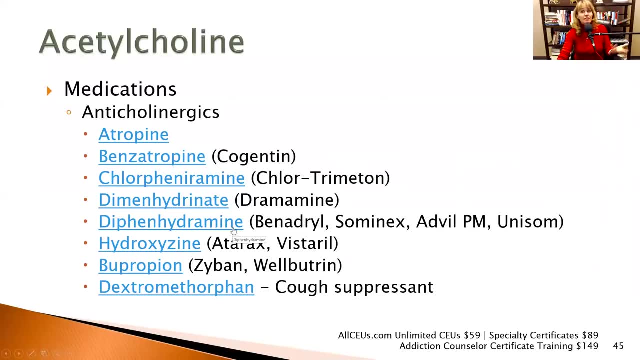 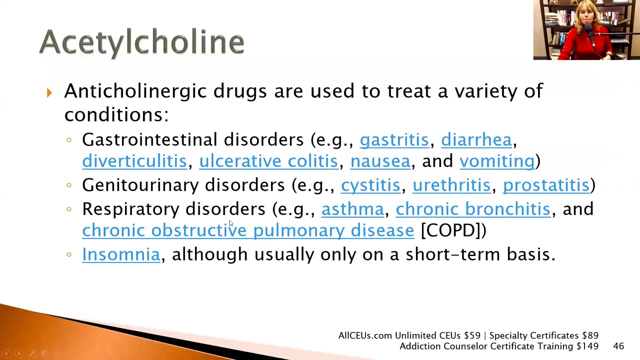 disorders such as chronic bronchitis and COPD, something else we see in older adults especially- and possibly insomnia, Usually only on a short-term basis. So going back to these drugs, thinking about what may be going on. diphenhydramine: not uncommon for insomnia on a short-term basis. 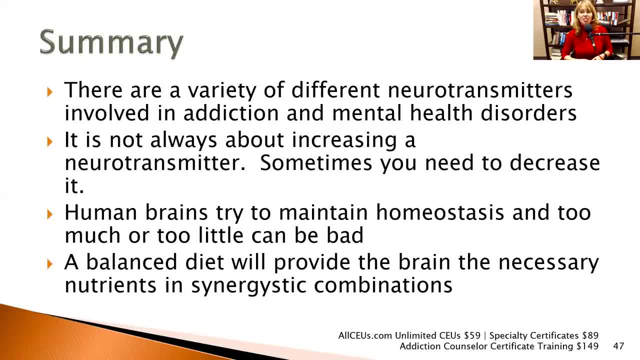 So there are a variety of different neurotransmitters involved in addiction and mental health disorders. It's not always about increasing a neurotransmitter. Sometimes you need to decrease it. The human brain tries to maintain homeostasis And too much or too little can be bad. If you think about it, I mean let's go back. 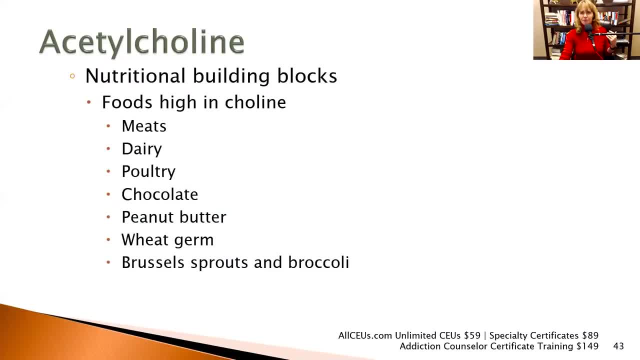 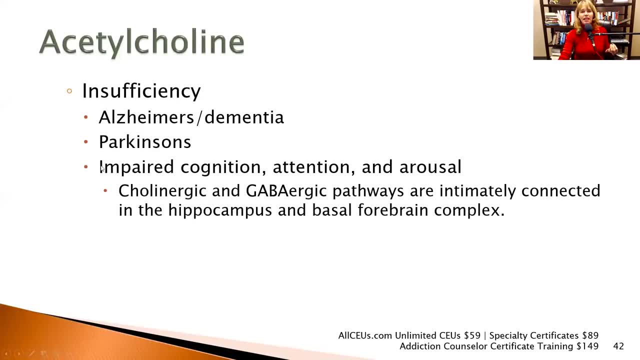 to acetylcholine for a second, if I can get there. How many of the neurotransmitters did we talk about today that, either an insufficiency or an excess, impairs cognition, attention and arousal? Pretty much every single one of them. So the cause of your client's depressive 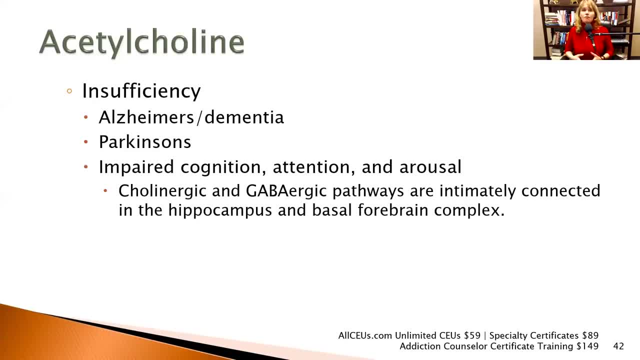 symptoms or anxiety symptoms, were really good at, you know, theoretically, at helping them figure out the cognitive distortions that may be contributing to turning on their threat response system or maintaining their depression. But as far as what, neurochemicals might be out of whack, especially for somebody who 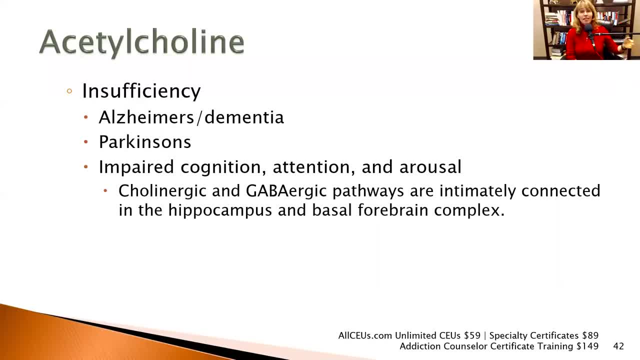 appears to have longstanding, organically involved depression. it's not situational, but they've had depression since they were, you know, in grade school. Well then, we want to look at what might be. where might a problem be in the plumbing, so to speak? Where might not enough of a particular neurotransmitter? 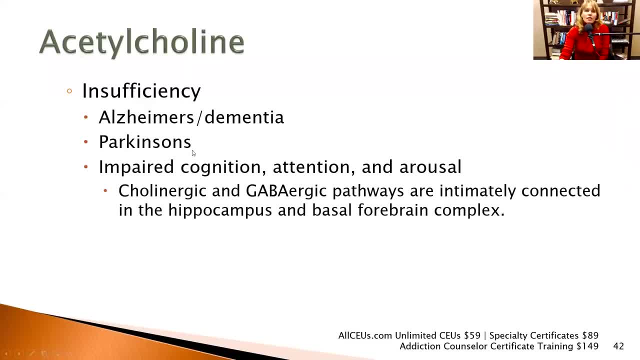 be getting through. This is something that a really awesome psychiatrist is going to help them kind of sort through. But one of the things I do with my clients is I have a check sheet of the different symptoms that they're experiencing And I encourage them. 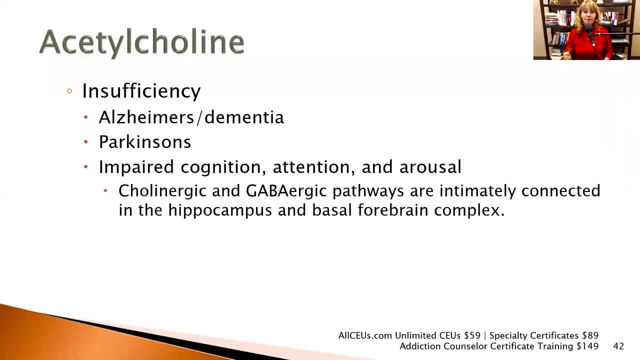 to keep track of their symptoms on a daily basis, especially if they're working with a doctor trying to get on a good medication regime for them, Identify when they start taking this medication, if there are side effects, if it starts helping them feel better, and anything that they want to talk with the doctor about so they 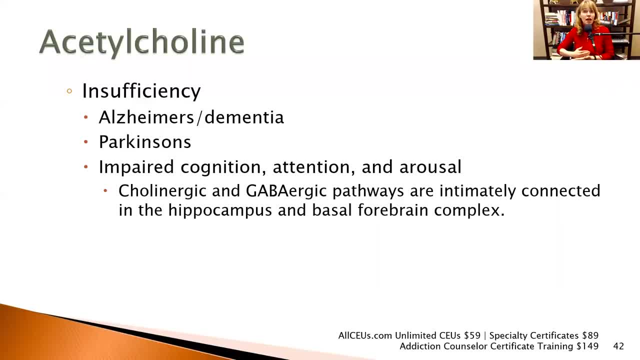 can figure out if they put them on a SNRI, a selective norepinephrine reuptake inhibitor. If they put them on that and that just makes them feel anxious as all get out, then they may try an SSRI or something else. 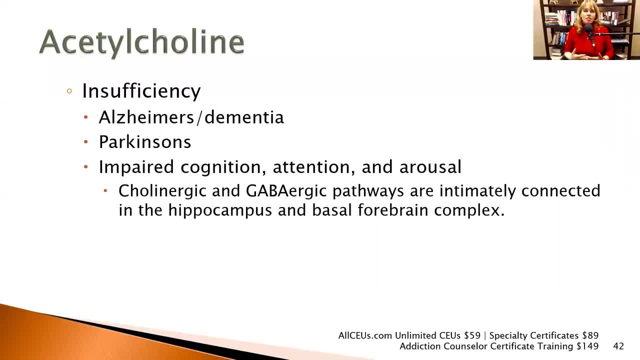 But it's sort of the whittling down which is some of our clients we see with treatment- resistant depression, as they call it. The doctors often wait until they've tried three or four or seven other things before they start looking at Seroquil and some of your ATP. 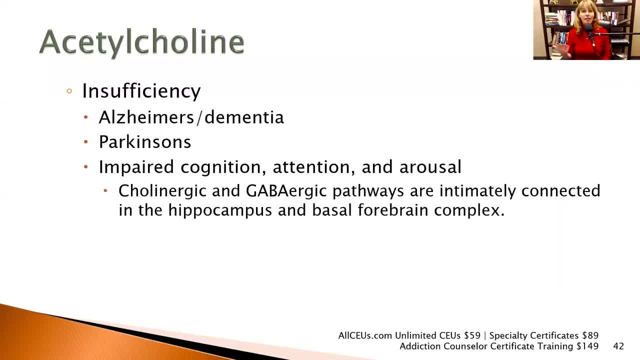 And I can understand why I mean. Seroquil is extremely sedating and does have some side effects. However, for some people, it may be a matter of getting the dopamine system back online, So encouraging clients not to give up, to recognize that, unfortunately- and I had this- 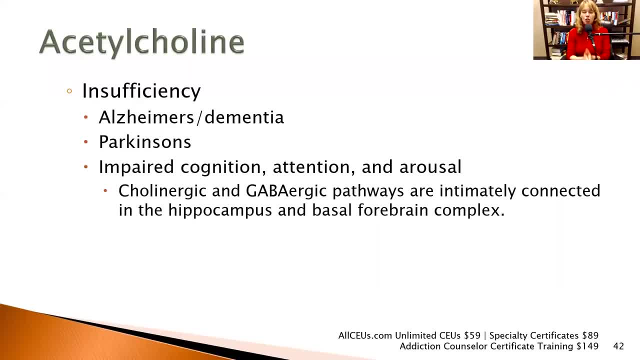 question come up when I taught this class before: there is no way to measure neurotransmitters in your brain while you are alive. So people who advertise that you can measure your neurotransmitters through your blood or your urine or whatever- yes, you can. 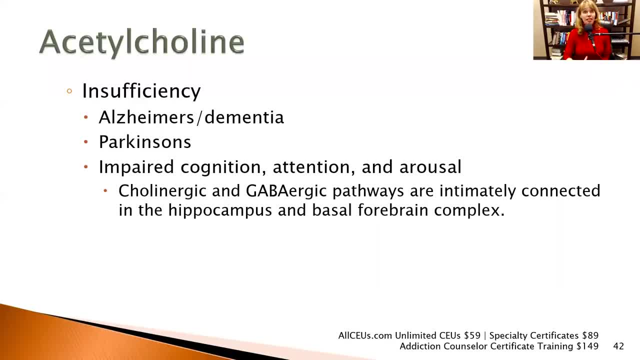 But what you're measuring is free circulating neurotransmitters. Remember I said, 80% of your serotonin is in your gut. Well, that doesn't do your mood any good. Well, except for when your belly doesn't hurt. But that number is really irrelevant. 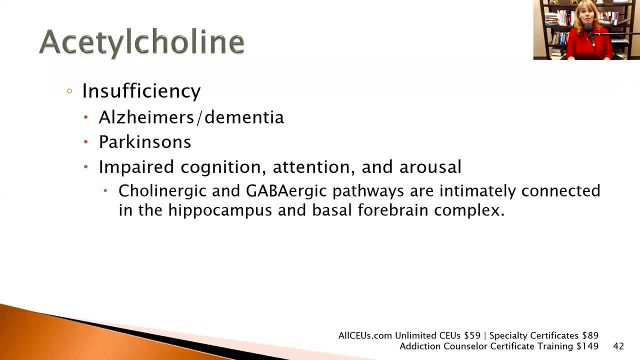 Relevant to helping doctors figure out which neurotransmitters might be precipitating mood symptoms. So it's a waste of money. I mean, people can do it if they want. you know, no harm, no foul. You also have the possibility of a placebo effect. 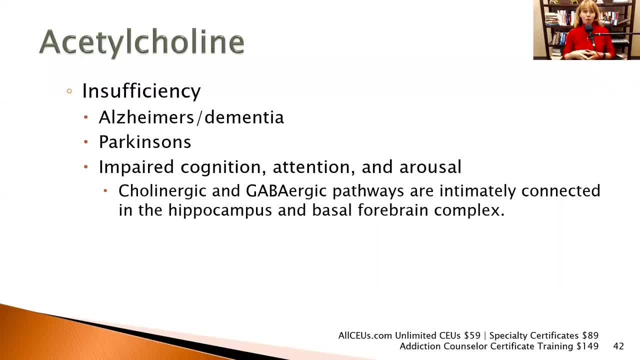 But in reality, there is no way that we have right now, at least that I'm aware of, to measure the actual levels of the neurotransmitters specifically in the brain. Uh so, Um, encouraging clients- and I use a much less technical presentation when I, when I 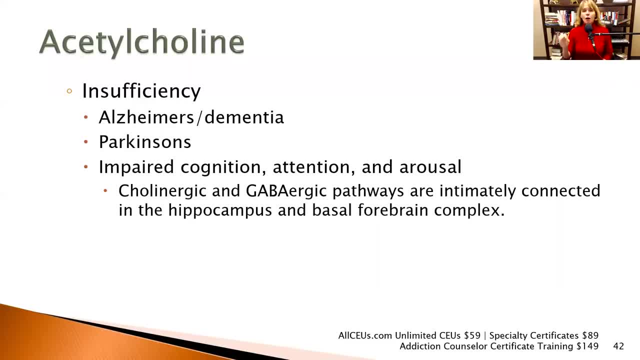 go through it with with clients and I do the mind body connection, but helping clients see how important it is to eat decently. you know pizza's fine, you know, a couple of times a week, even if that's what you want, but you need to get some of that brown rice. 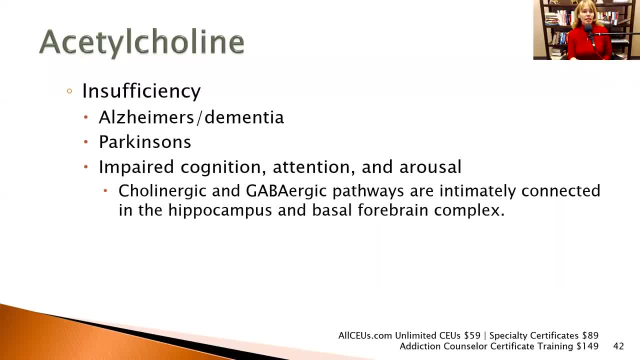 and vegetables and other things. When we start thinking about some of our clients who are going on The Indie nutritional plans um, where they're cutting out all grains, you know: no rice, no wheat, no oats, no nothing. 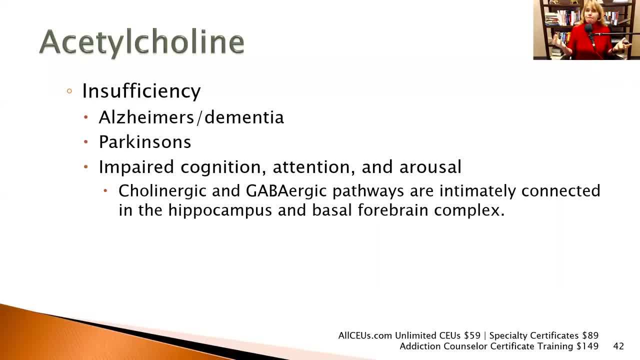 Um, and they're just eating meat and vegetables. What impact is that having on the availability of neurotransmitters, Since most of these neurotransmitters can be formed from building blocks that are found in green leafy vegetables or, um, your grains, as long as they're getting a fair amount of? 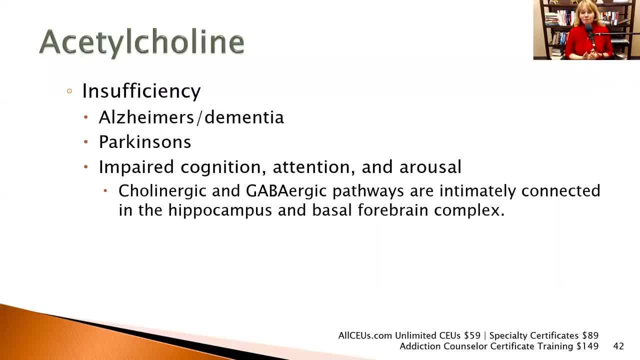 green leafy vegetables. They're probably going to be okay. But you know again, once you start monkeying with cutting out entire food groups, it can cause unexpected side effects. Um, so making sure that clients are aware of that, not saying not to do it, they're. 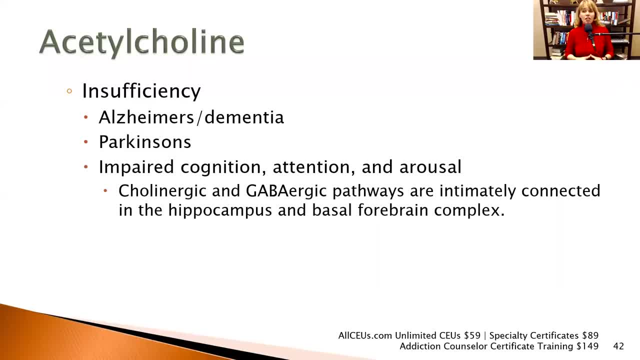 going to do whatever they want to do, Um, but encouraging them to talk it over with their doctor and and or a nutritionist- And I always say a nutritionist, but most of them, well, I haven't yet had a client that has actually gone to see one. um, because they 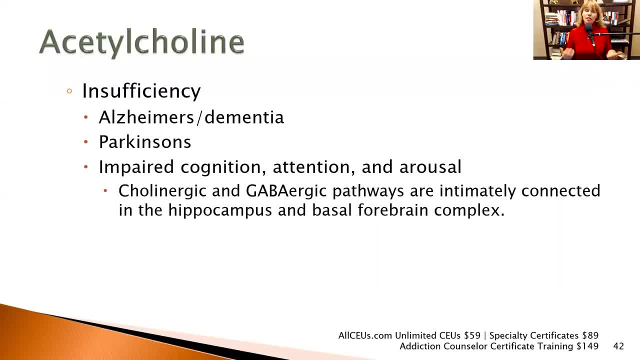 kind of roll their eyes and they go: well, that's not covered by insurance, And well, uh. so at least talk about it with your doctor before you start monkeying with things, just to make sure that you're not going to make anything worse. 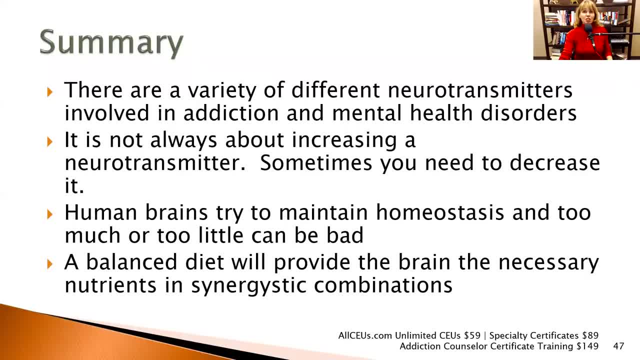 Human brains try to maintain homeostasis. too much or too little can be bad, And a balanced diet will provide the brain the necessary nutrients in synergistic combinations, And that's something I didn't talk about earlier. Taking a pill is not a substitute for eating, you know, nutritionally balanced foods, because 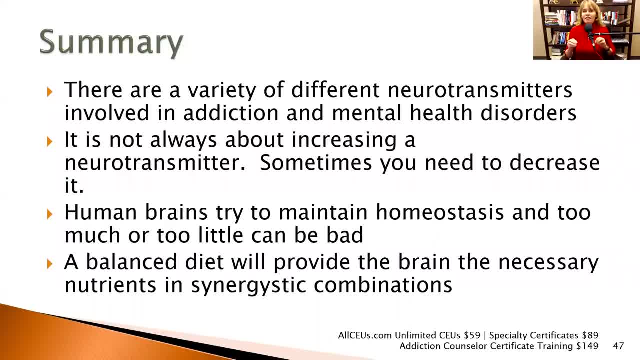 those amino acids, for example, are in a very specific ratio in terms of what's absorbable. I will give you an example. We think of Turkey and Thanksgiving and we think, well, Turkey's high in tryptophan. So when I eat Turkey I get sleepy and it's it's because of the tryptophan and the Turkey. 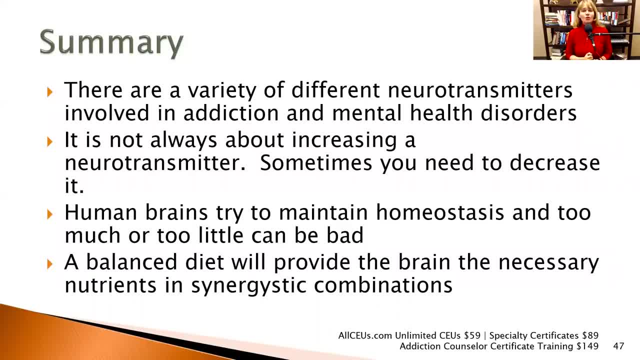 research has actually shown that that's not true. Research has shown that, yes, Turkey does have a high amount of tryptophan, but it also has a high amount of other amino acids that are preferred by your body, So you don't get very much actual tryptophan synthesized when you eat Turkey. 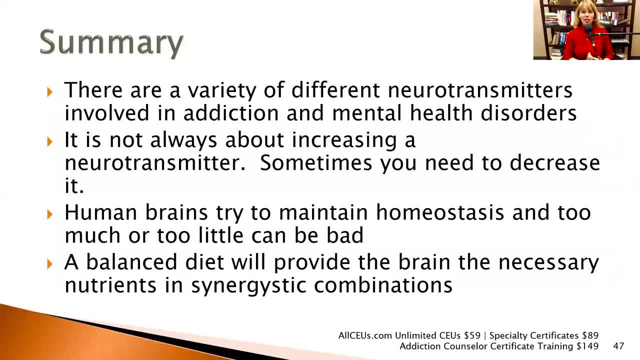 So they hypothesize that it's actually the sugar crash from the sweet potatoes and everybody, everything. As opposed to Turkey, chicken is actually higher in available tryptophan than Turkey is. So these little things that you know people don't don't take into consideration necessarily. 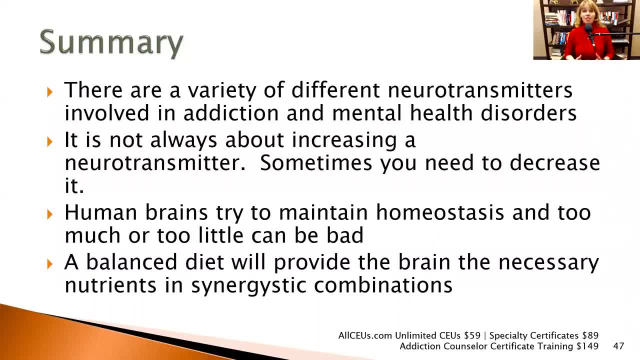 and they can get obsessive about it, trying to figure out, you know, micronutrients and proteins and amino acids and everything down to the nth degree And it's really talking to- I'm a dietician friend of mine- is it's really not that necessary? 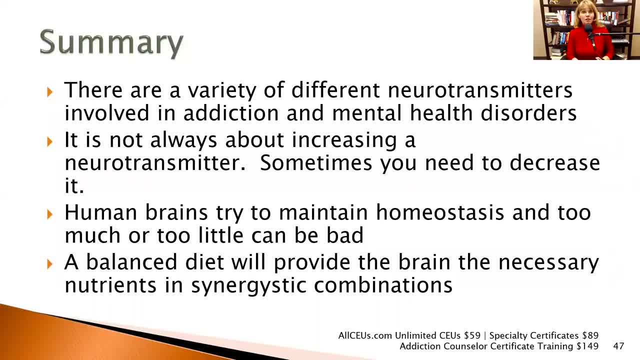 If you eat three colors on your plate at every meal. you know you can have fruit at breakfast, because most of us don't want to eat Brussels sprouts at breakfast- and and you eat enough calories and you eat quality foods. you know pizza has a lot of colors, but that doesn't. 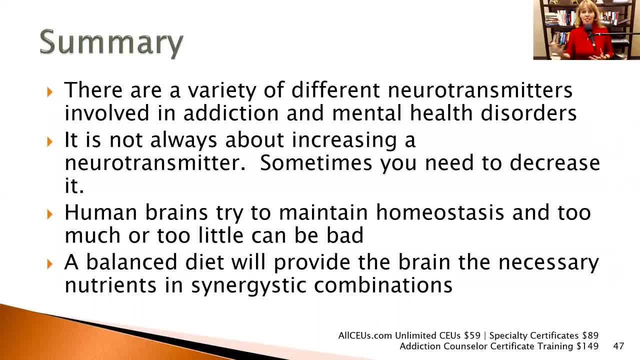 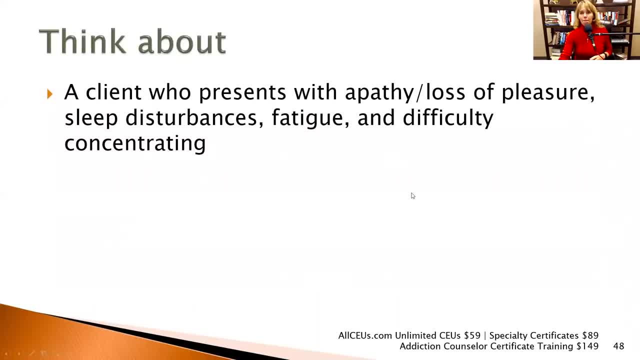 count, as you know, a well-rounded meal for every single meal, then you're probably going to get adequate nutrition. Are there questions- And I will look up that question- about Wellbutrin as a dopamine agonist? I just don't know the answer to that. 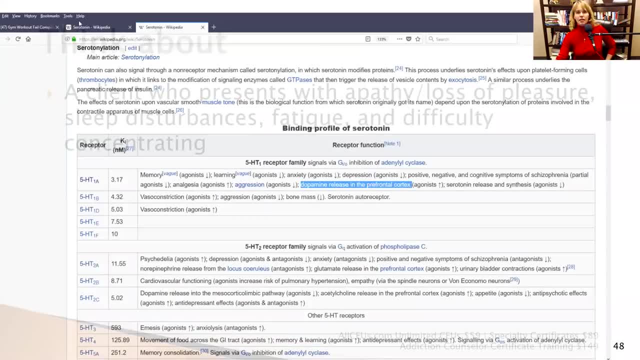 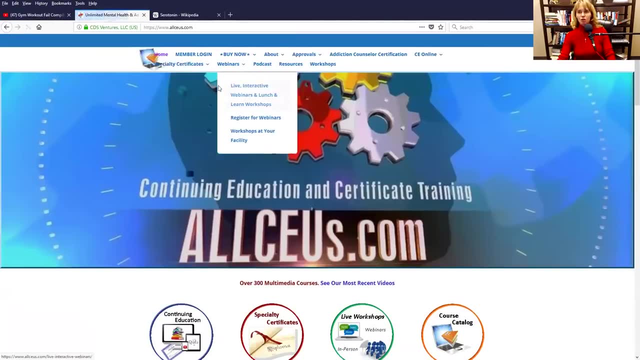 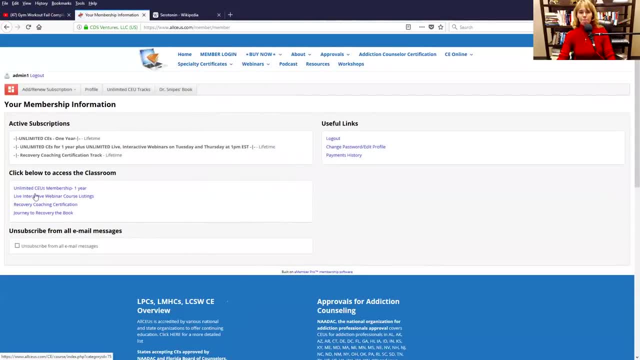 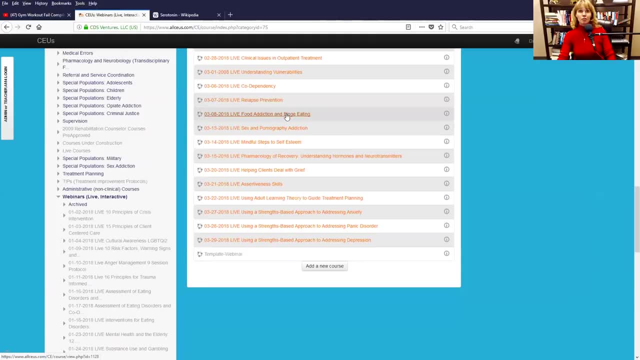 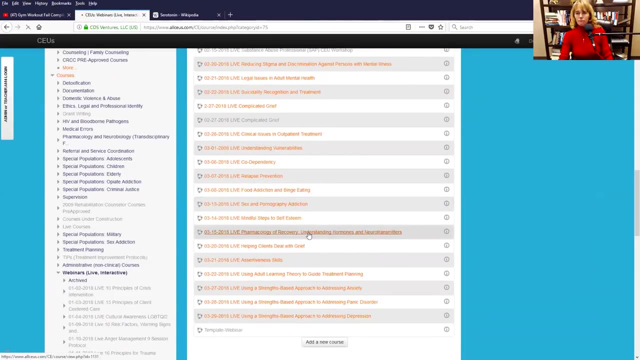 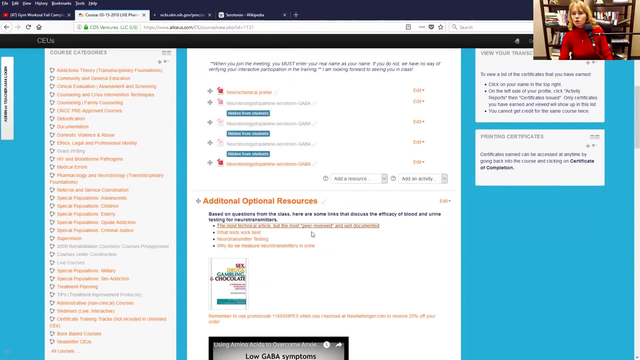 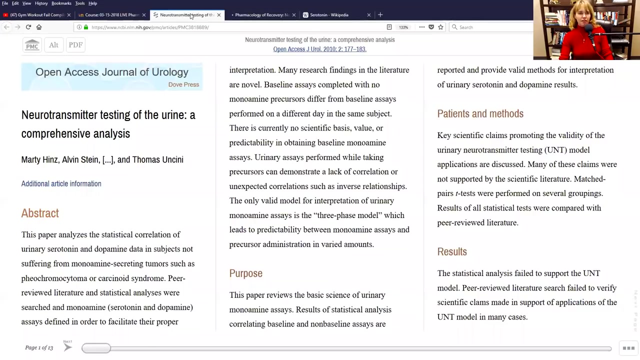 That goes over all the neurotransmitters. So if you like reading that kind of stuff, it's a really awesome book. It's free, It's online. Let's see. Let's see what we have here. Okay, One of the slides at the end suggested it. 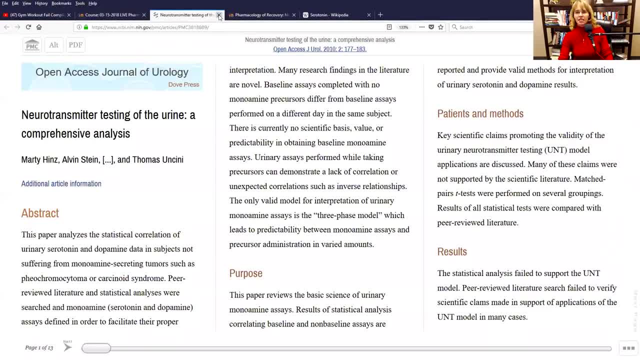 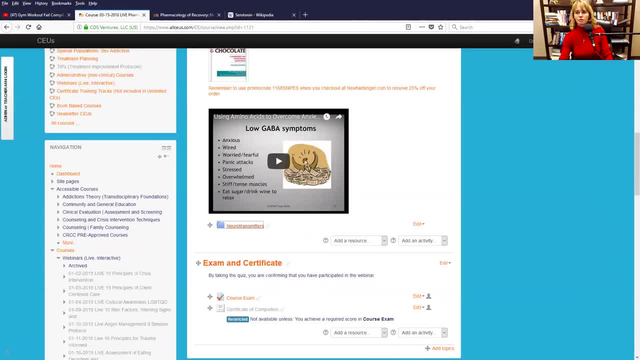 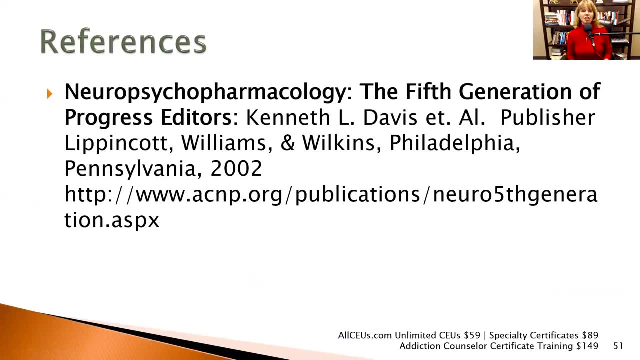 Hey, cool, That's not it. Okay, So let's go back here. Yes, Thank you, Carl. Neuropsychopharmacology: the fifth generation of progress. Editors Kenneth L Davis et al. This link will take you directly to it. 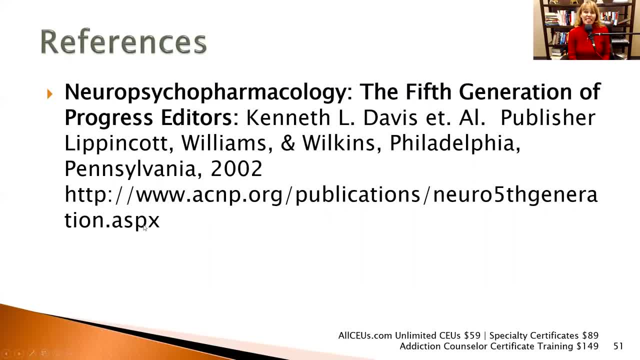 Oops, And I love it. It is written in, you know, journalese, So it's not something that you want to plan on sitting down and reading 100 pages at a time, Because you'll probably go cross-eyed, But it is a fascinating read. 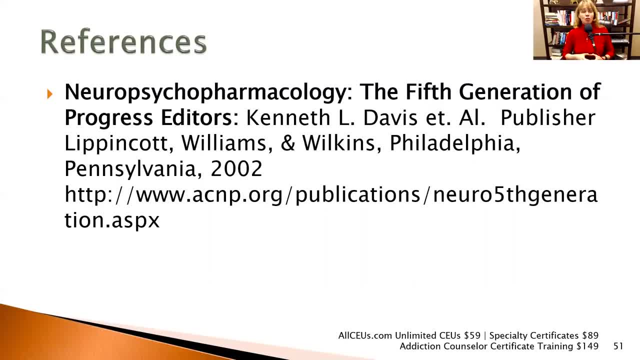 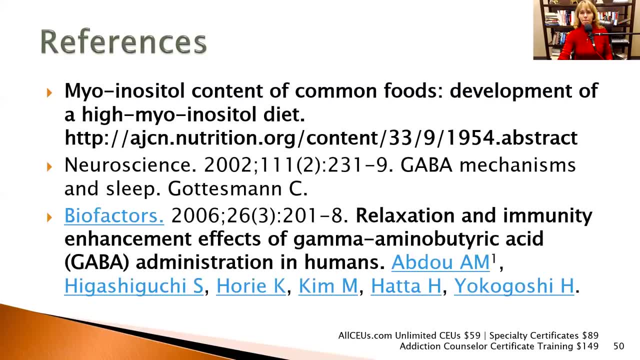 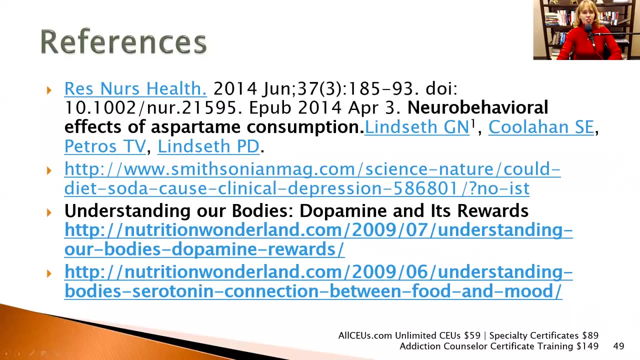 And it does kind of break down each individual neurotransmitter to help you get an idea about you know what it does. And then some of the other articles I just found very interesting in terms of increasing our understanding and increasing our clients' understanding of neurotransmitters. 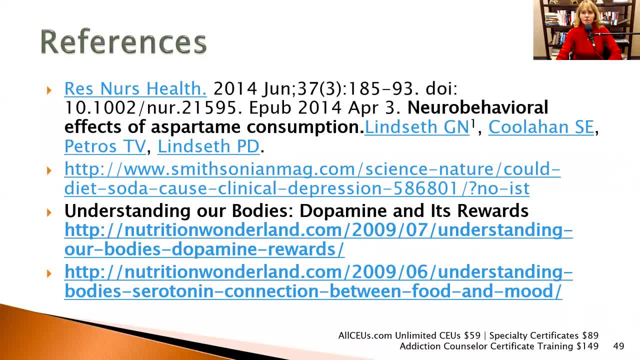 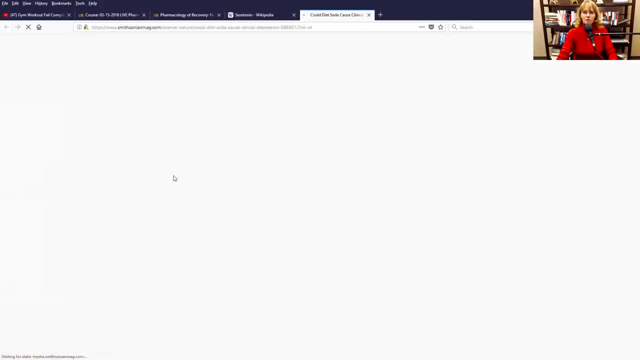 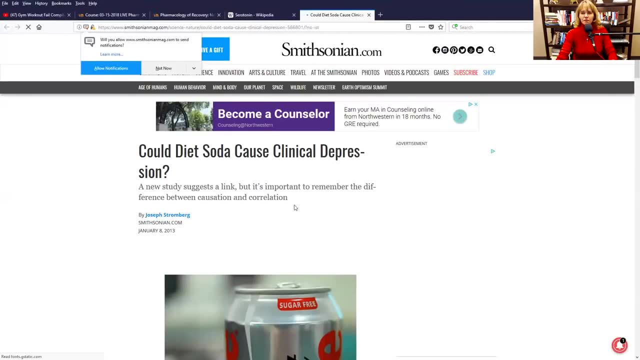 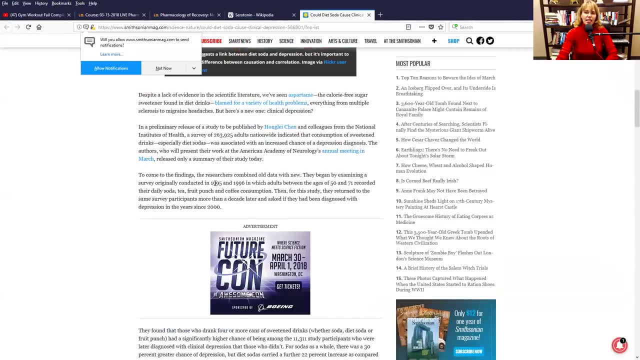 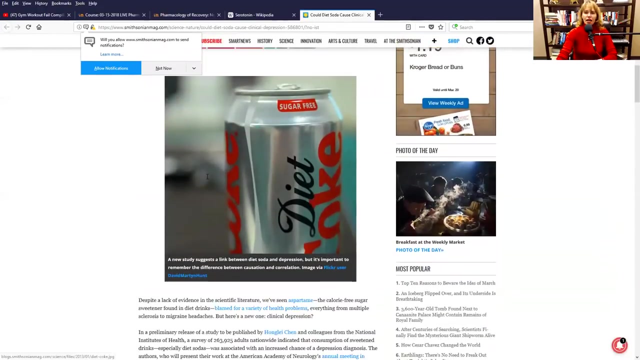 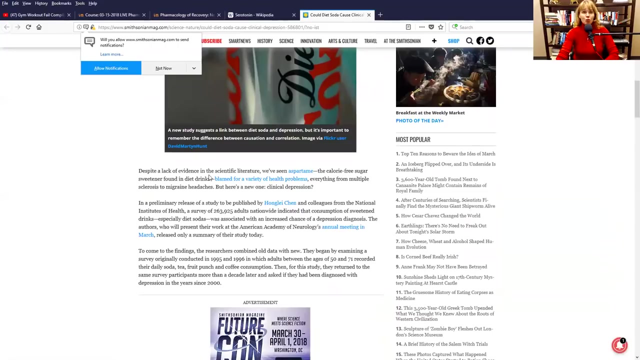 I did like this study- And it's, you know, only tangentially related to the neurotransmitters- about whether diet soda causes depression. depression because it really does talk about the difference between causation and correlation. Is there a correlation between depressive symptoms and low serotonin? Yes, Do we know. 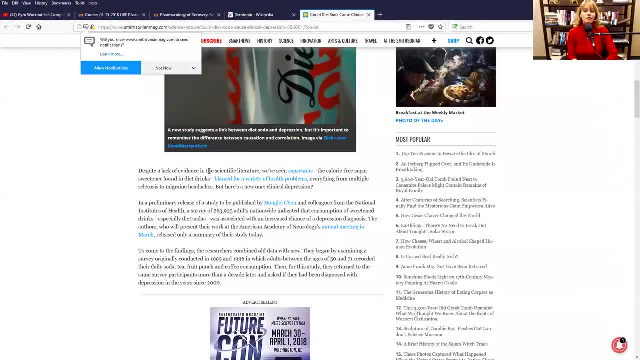 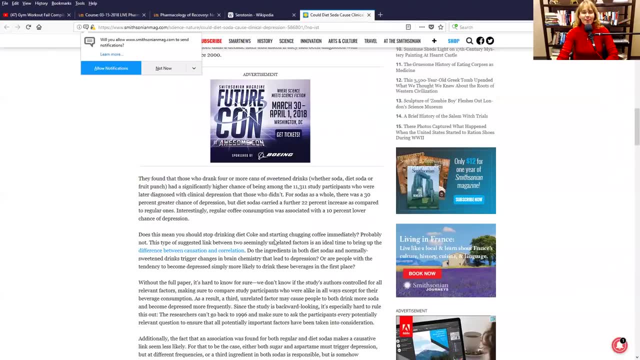 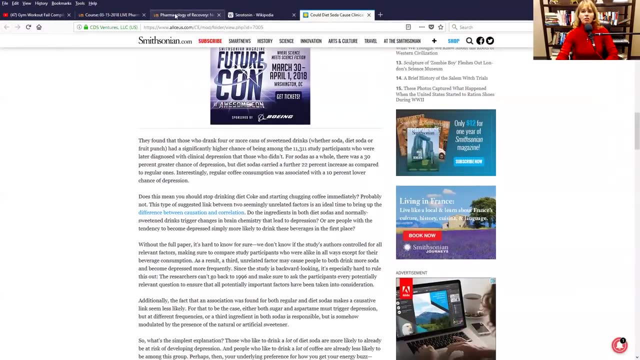 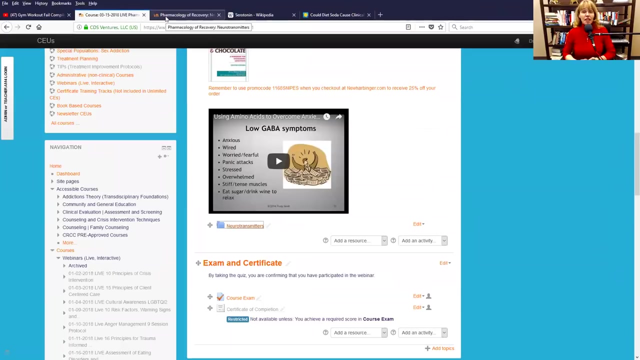 whether low serotonin causes depression. No, not necessarily. So we need to be cognizant of what other things might be causing these symptoms, And we talked a lot today about neurochemical imbalances. but there are a ton of physical things like just even hypo or hyper. 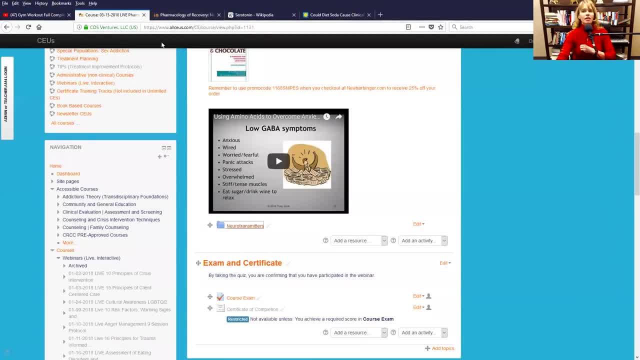 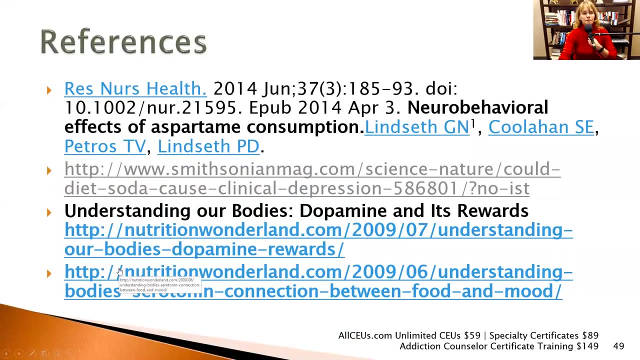 thyroid or imbalances in sex hormones that can cause fatigue, difficulty concentrating, low libido, apathy. So we don't want to assume necessarily All righty. If there are no other questions, then I will look up that one thing and I will put that.